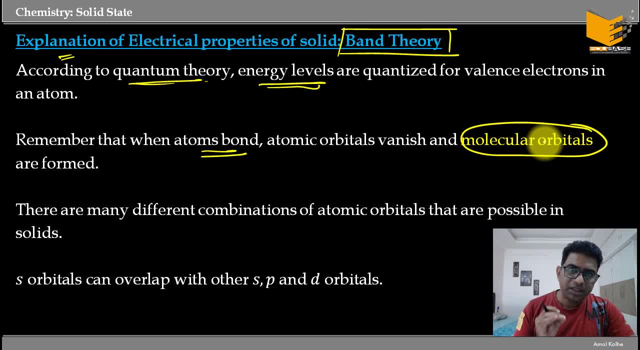 here. basically, Okay, the same concept of quantum theory. We will tell you about everything else. So you are aware of bonding and anti-bonding orbital. Here we are just going to use the terms separately. Okay, so there are different combinations When the atomic orbitals are being combined. okay, so different combinations. 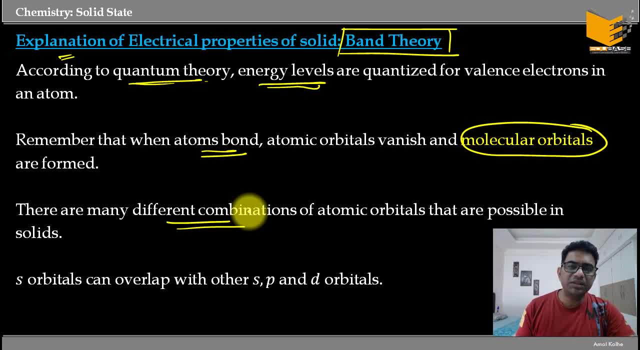 can be possible. Okay, And we call the possibility of impossible something like band. Basically you get a kind of like a band which we will see in a little while. So the overlap of orbitals also can be seen in covalent or non-covalent compounds. But we are going to explain in. 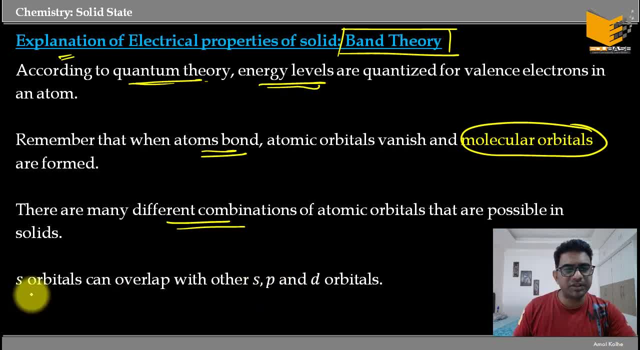 orbitals that can have many different possible combinations. for example, s orbital can overlap with other s, p and d orbital, so one atom s orbital can overlap with other s, p and d orbital, so there are different number of combinations that are possible. so what happens is that 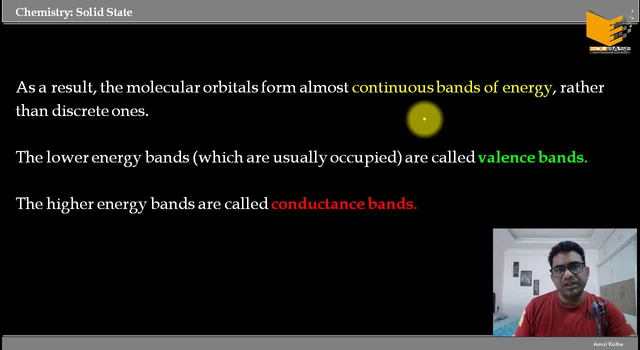 if we look at metal or any covalent compound, then there are lot of metal atoms, isn't it? there are lot of metal atoms and in every metal atom there are orbitals or orbits, which we call. we don't actually use orbit as a term, we use orbital. so there are orbitals and in 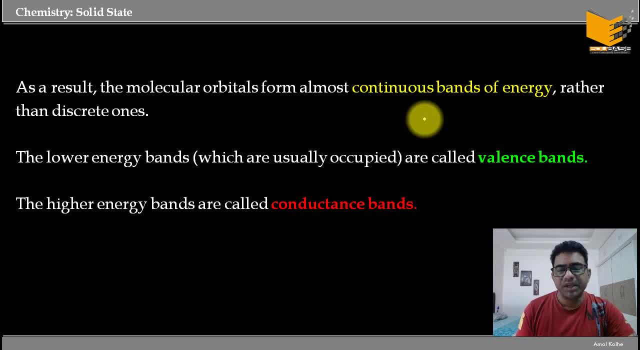 those orbitals there are electrons. ok, so when two atoms orbitals overlap, then what we get is a continuous band of energy. ok, because there are lot of orbitals, and when lot of orbitals are overlap, the permutations will be there. so what we get is a continuous band of energy. 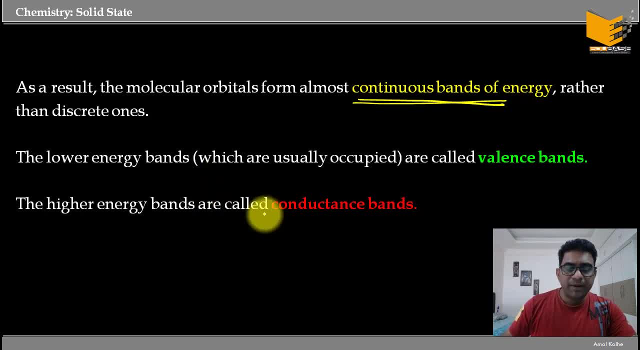 level, ok, this becomes a continuous band, and here we are not getting a discrete band. if we talk about atomic orbital, then these are discrete levels, ok. but in molecule orbital, ok, get a continuous energy bands. ok, so the lower energy bands are called valence bands, ok, not. 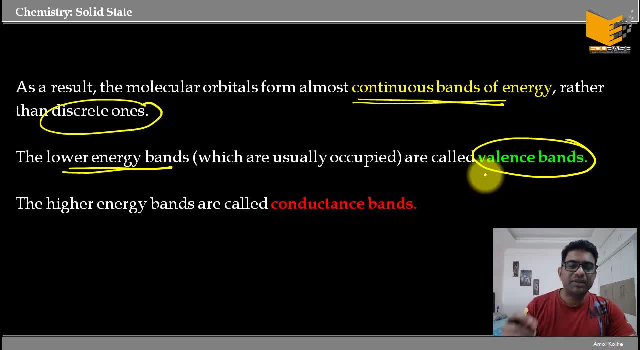 valence bond. it's. a valence band means this is similar to bonding orbital. ok, the lower energy ones are called valence bands. see, we can't use orbital because there is no single orbital. it's a band of various orbitals, isn't it? that's why we are calling it a band, essentially. 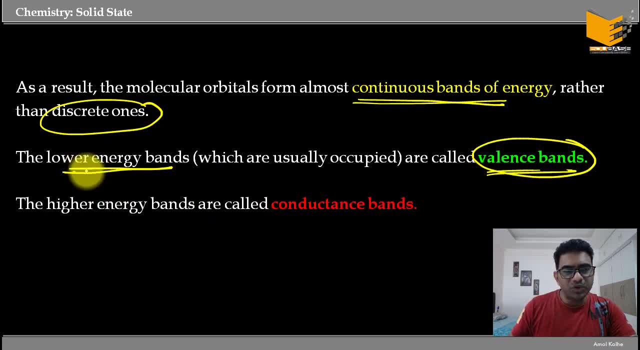 it's a band of energy, ok, so the lower energy one is called valence band and it's generally occupied. so valence band contains electrons- ok, and the higher energy one, which is similar to anti bonding, i can say, is called conductance band- ok, and it generally has no electrons. 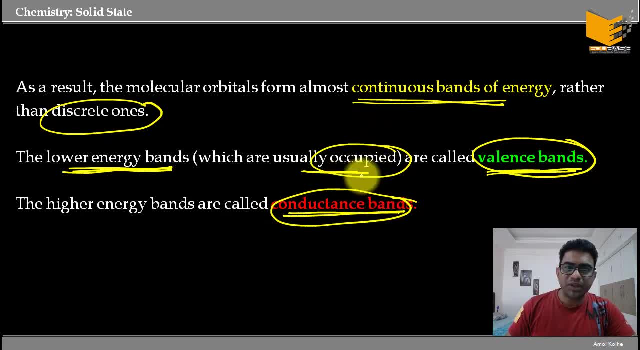 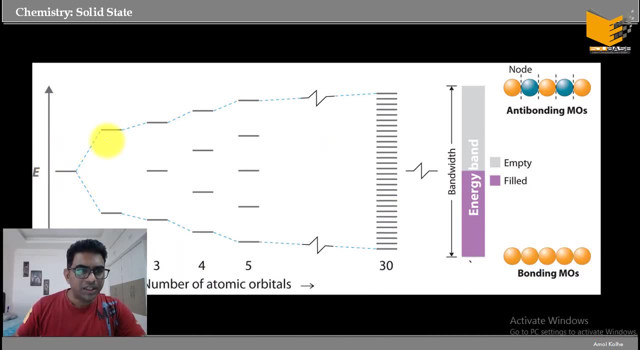 at least not at ground state. ok, so see electrons which are in ground state. they will remain in valence band and in conductance band. generally. electrons will not remain, or may be some electrons will be there. So I show you this diagrammatically. so if two atoms are combined, then we will get a. 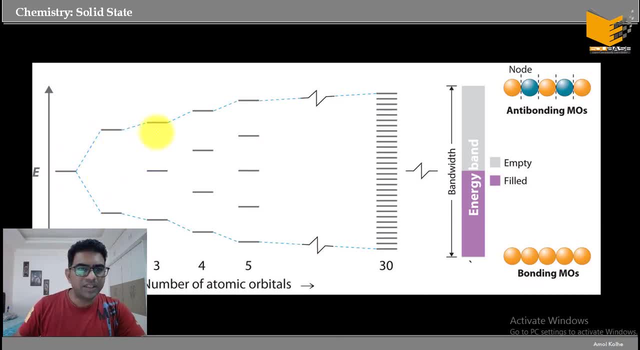 possibility that in this way we will get two overlaps. if three orbitals are overlapping, then in this way, if four are happening in this way, if five are happening in this way, you can see the gaps are getting filled. If there is a lot of number of like, if we are taking 30 bands, if 30 orbitals are overlapping. 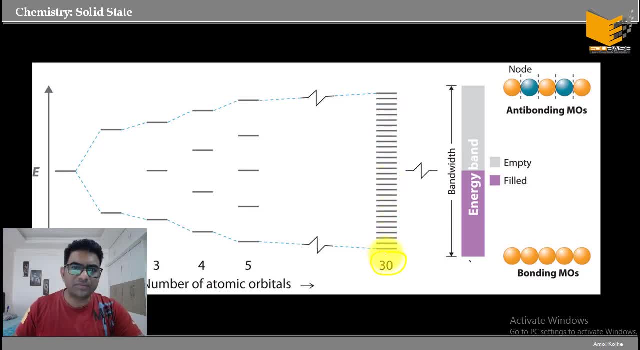 then you can see almost a band is getting formed. This is not a continuous band, but almost all the things are filled. But if you have infinite number of orbitals, because there are billions and billions of atoms and their orbitals and their orbitals are overlapping, then ultimately what we will 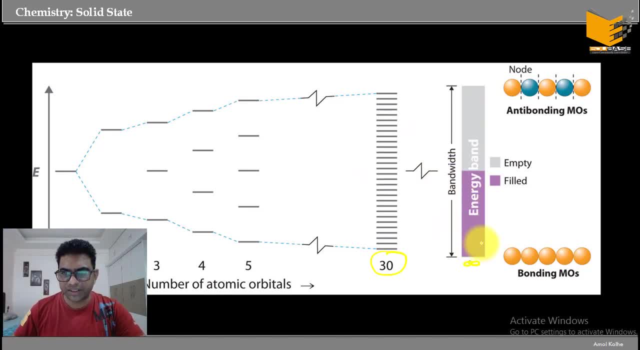 get. We will get a continuous band which we are calling this. This is the band And the lower portion in which electrons will be there. we will call it valence band. So this is your valence band. Now, this is formed because of the bonding molecular orbitals. 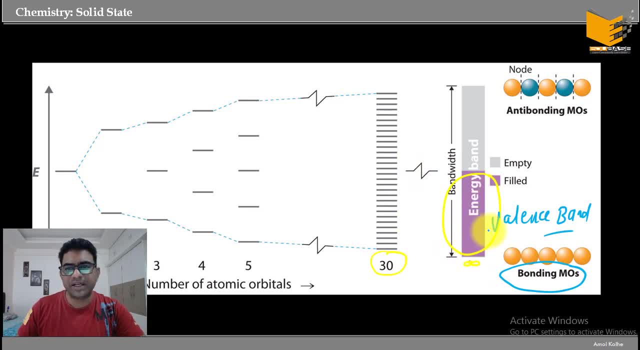 Because of that, we are getting valence band in which electrons will be there, And next is this band. We call this conduction band. We call this as conductance band, Conductance band. This is similar to anti bonding orbital. ok. 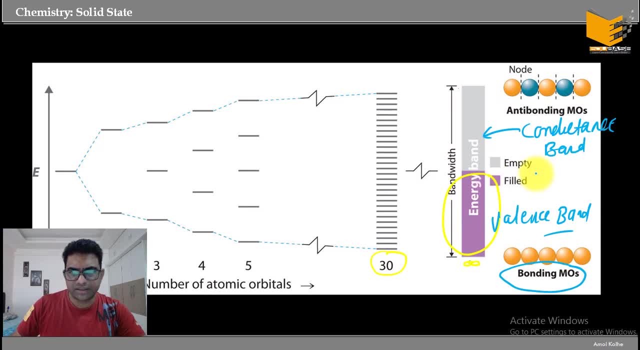 So here electrons will not be there. This is what we imagine. So essentially, if you see here valence band and conductance band are almost connected, Isn't it? This is happening. It can also happen that valence band, if you assume this, is valence band, ok. 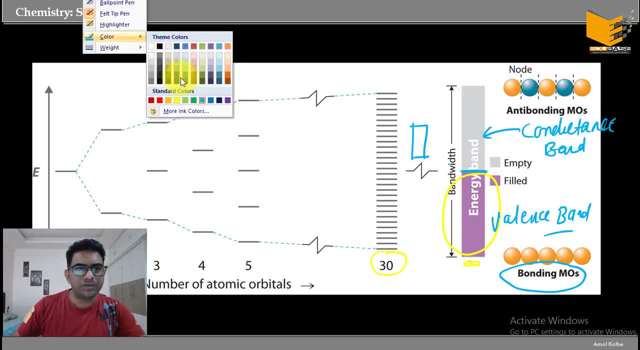 So conductance band can overlap, so I will use a different color for that, let's say conductance band. so this can also be a situation, or it can also be that valence band and conductance band are separated by some distance. that is also possible. it will depend on what kind of orbital we are overlapping. 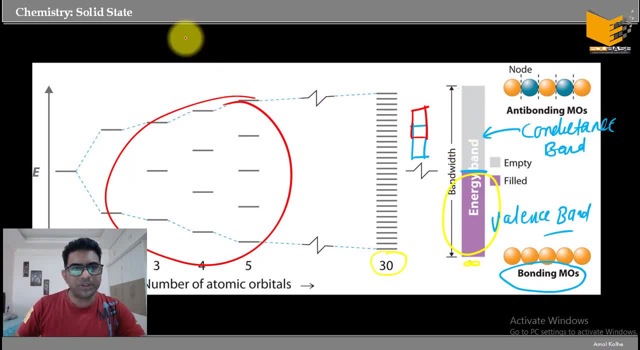 so we basically have three possibilities. one possibility will be that the band is connected. the second possibility is we will go with four possibilities. the second possibility is that the bands are overlapping. third possibility is that there is a gap in between the two bands. 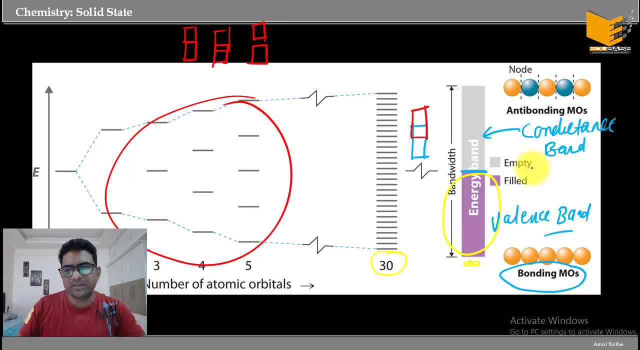 valence band on the upper and conductance band on the top. that is how it is. And the fourth possibility is that there is a gap between two of the bands. that means This gap is called forbidden gap or forbidden band. Electrons can't be here. they can either be here or up. 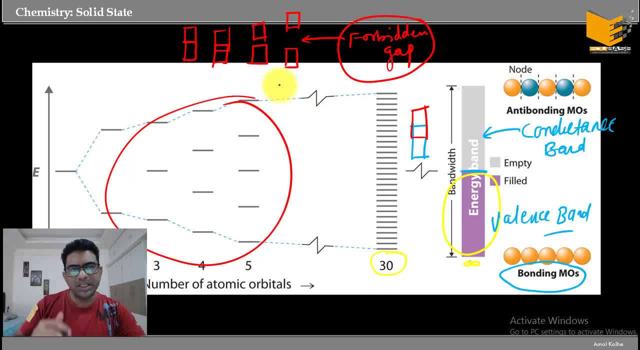 As we have seen, electrons are present in anti-bonding orbitals and their bonding order is degrees. We have seen this in molecular orbital theory, So we are using a similar concept here, But because we are seeing a lot of overlap of orbitals here. 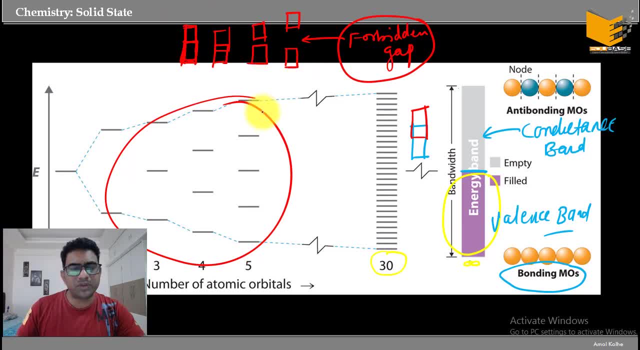 so we get a valence band and a conduction band and it has four possibilities. Let's consider these two possibilities as one. This is one, this is two and this is three. So let's assume that they are either touching or overlapping. 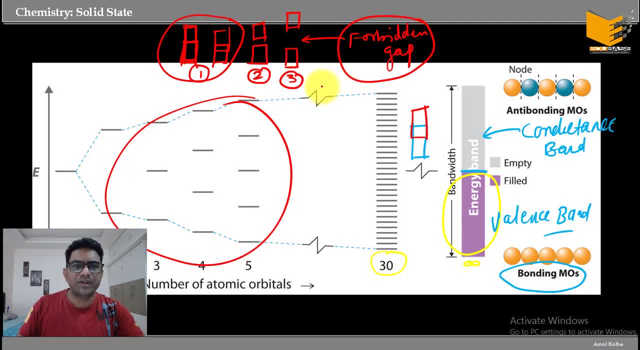 This is one possibility. Secondly, it has a little gap. And the third possibility is that there is a lot of gap between these two bands Understood. So we are getting these possibilities. This possibility is the valence band and the conduction band are overlapping or touching. 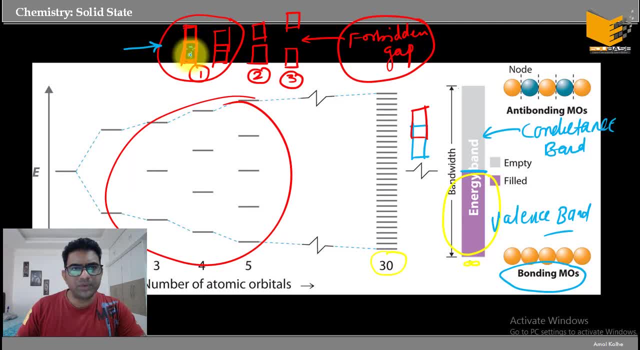 So this means if electrons are present in valence band, we are saying that electrons will remain in valence band and not in conduction bands. But it is possible that electrons will go to conduction band from valence band because there is absolutely no gap in there. 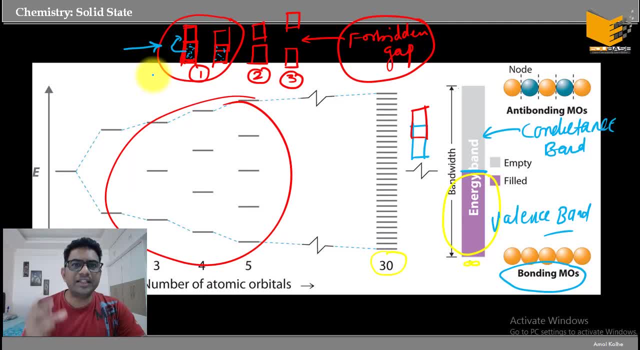 There is no difference. If we say gap, then this is basically like an energy barrier. Okay, So this energy and this energy. there is no energy barrier between them. So electrons from valence band can easily go to the conduction band. 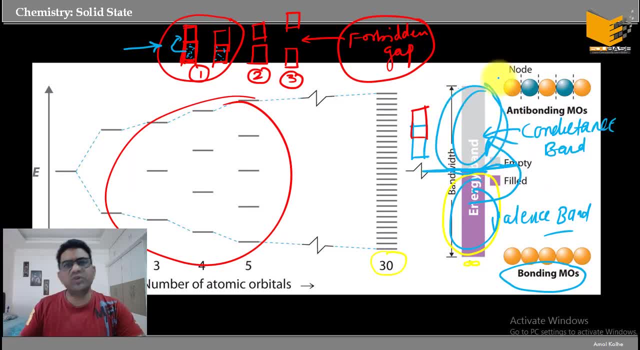 And when electrons come in conduction band, then we get conductivity. Okay, If electrons are only in valence band, then these are bound electrons. Okay, These are electrons between two atoms, That is, electrons between the molecular orbital. So these electrons are generally considered immobile. 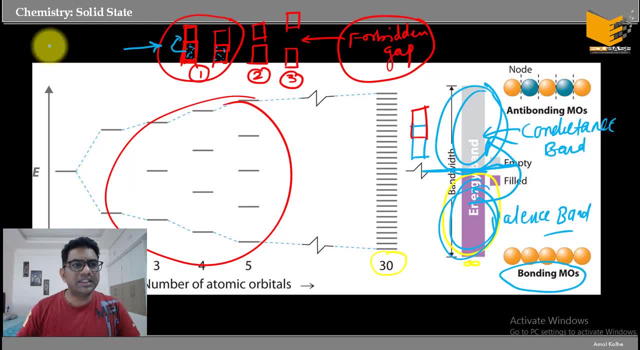 This means that we will not get conductivity. So this is basically something that is forming a covalent bond. Okay, So if I am taking hydrogen, then these electrons between two atoms will remain in valence band, Isn't it? And if electrons come in conduction band, that is, in the upper level, then we will get conductivity. 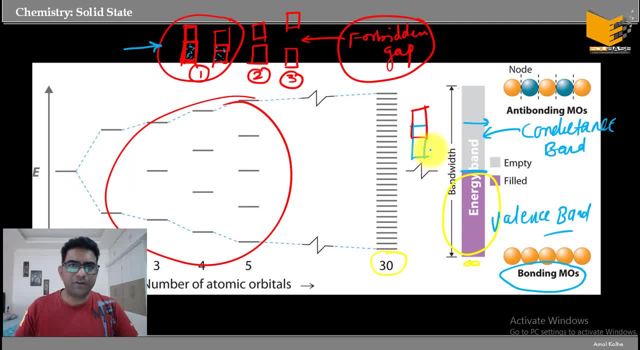 So these electrons will remain mobile. So these electrons will remain free For mobility. Now, in the case of covalent bond, if you realize that we will have to break electrons, we will have to break bonds, then only electrons can be free. 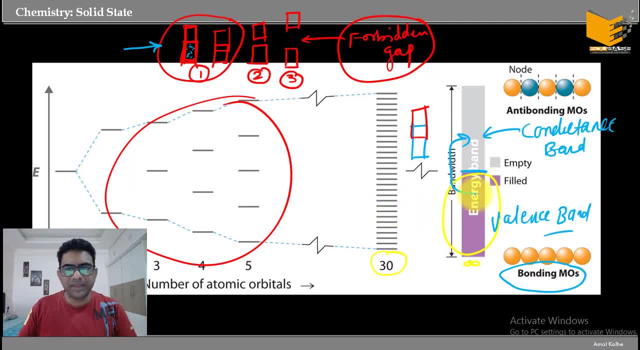 Isn't it? But in the case of metals that is not the case. In the case of metals, electrons can easily go from valence band to conduction band, And when they come in conduction band then you get conductivity Okay. 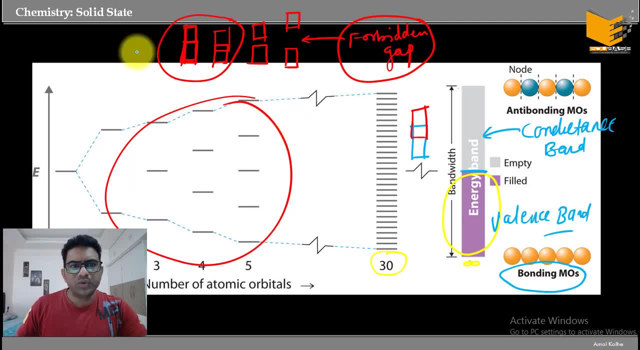 So this is how we have to visualize it. All right, So the point here is this: Okay, When electrons go from valence band to conduction band, then only we will get conductivity, Otherwise we will not get. So now look at this situation. 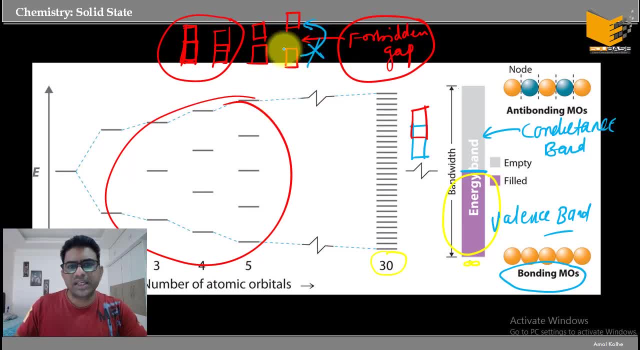 Can electrons go from here to conduction band? They cannot go Because the energy gap between the two bands is very large. We cannot provide so much energy that the electrons go from here to here. Okay, So what? we will get here Here. 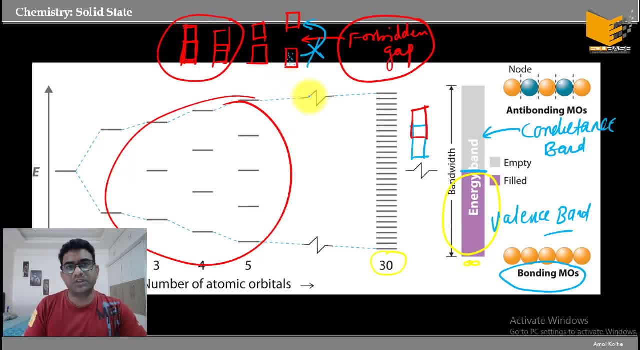 Where we have to make sure that the electrons are in the right place. Now I am telling you that this is a very simple situation. This is a very simple situation, All right. It will be obvious that in these conditions, the conductivity will be very less or not. 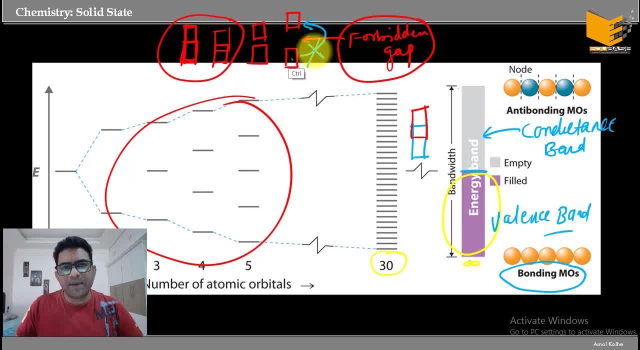 at all. That is also possible, As I have mentioned that a little bit of conductivity is available to us, All right, So maybe a few electrons will always be there, but the conductivity that is negligible, it will be neglected. So this situation will be with Insulator. 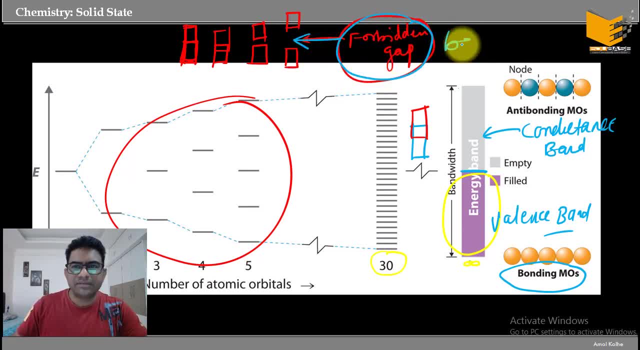 Understand. So this gap is coming. Okay, This gap is coming. What we are calling it forbidden gap or forbidden band also. this is also forbidden band. there is no forbidden band here. okay, here is forbidden band and here is forbidden band. so electrons can't be here means it's not like electron. 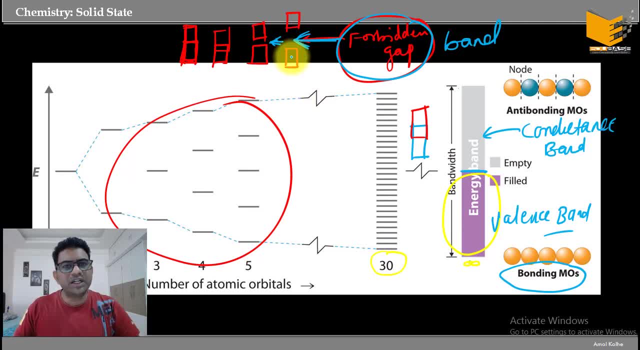 can travel. okay, electron can travel. electron can jump from here to here directly, but this gap can't go from there and this concept also emerges from quantum theory. basically, if you remember the quantum theory, molecular orbital theory in this also we said this started with bohr theory. to quantum theory we used to say that electrons can't be in between two orbital. 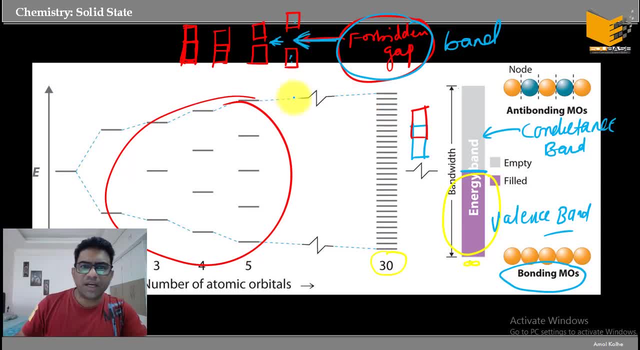 or orbitals. okay, so here also the same thing is coming. electrons can't be in between. electrons can be here and here. electrons will be here in ground state. if i provide energy, then electrons can go in higher state, and if they come here, then i will get conductivity. now 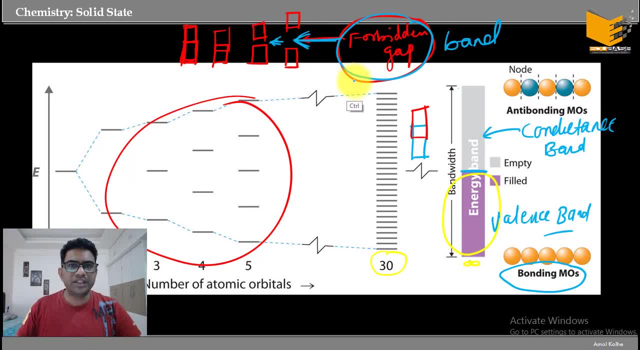 from this. only we distinguish between conductors, insulators and semiconductors. okay, so these three things we will see now. i will show you the conduction band. sorry, i will show you the bands of three substances and you will understand all these things. all right, see what is happening with. 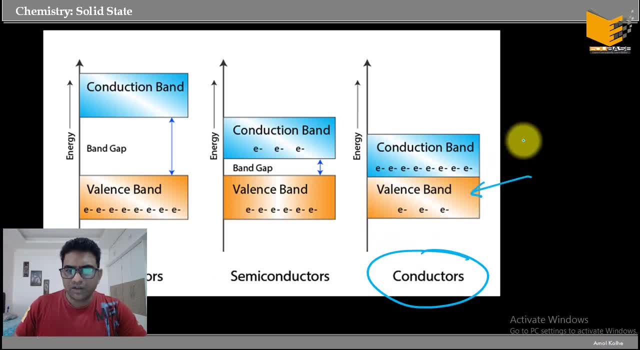 conductors. in conductors, you have a valence band and you have a conduction band. okay, and there is absolutely no gap between the two. okay, or it may also be that they are overlapping. okay, this portion may also be overlapping. so there is no gap between the conduction and 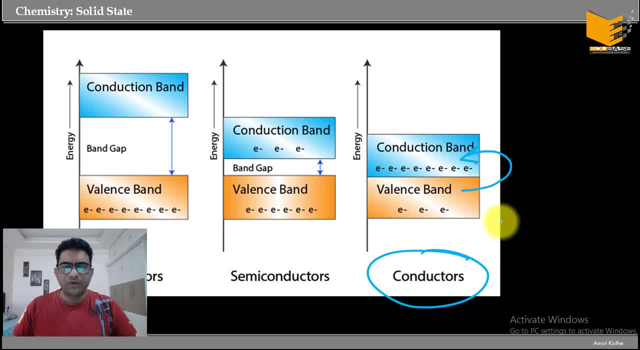 a valence band. so because of this electrons can go nicely from valence band to conduction band. there is absolutely no resistance for moment of electron from valence band to conduction band. resistance means that electrons can freely move into the conduction band and when they 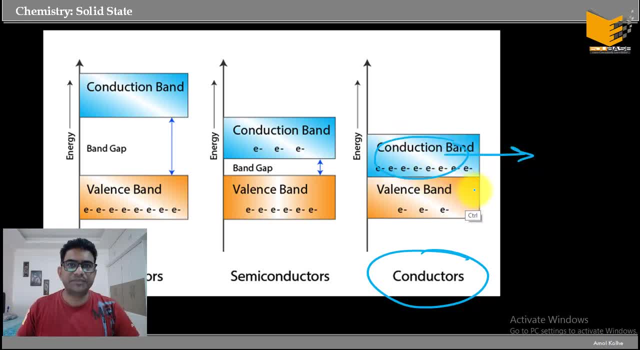 remain in conduction band, then we will get conductivity okay. so conductors are the ones. conductors are good conductors because there are lot of electrons in the valence band, isn't it? because of more electrons in the valence band their conductivity will be more. we have seen. 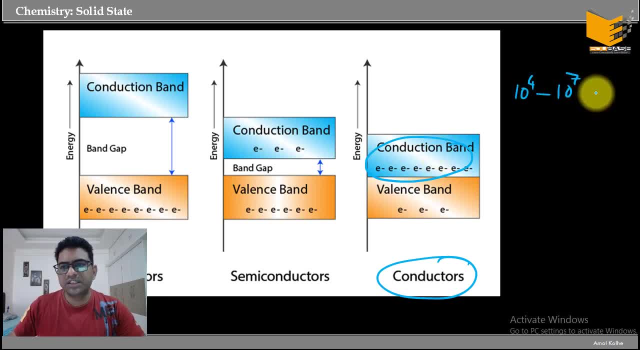 it is 10 to the power, 4 to 10 to the power, 7 siemens per meter. ok, or ohm per ohm per meter. we also write, and per ohm is basically siemens. so from 10 to the power, 4 to 10 to. 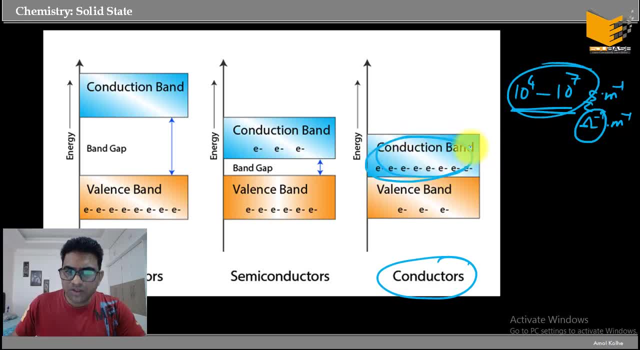 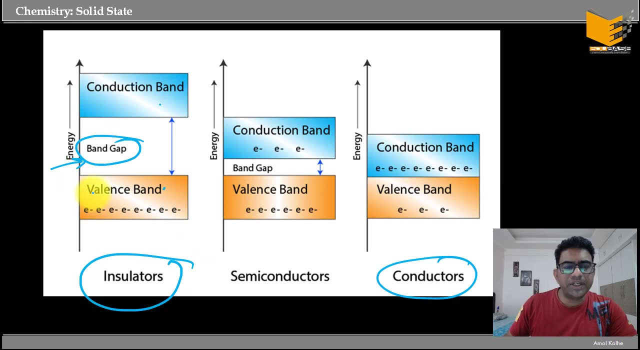 the power 7 we take conduction because there are lot of electrons here, so you can easily get conductivity. ok, now let's look at insulators. in insulators there is lot of gap. in valence band and conduction band it is called forbidden gap, forbidden band or band gap, whatever you. 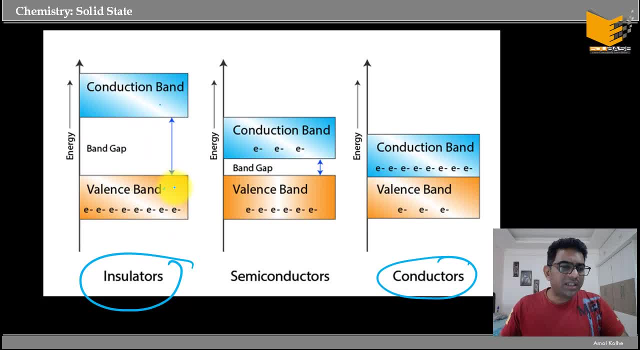 want to call it, you can call it. alright, from here to here. it is almost impossible. it is not impossible, it is almost impossible, it is almost impossible. we can't give so much energy at any given point, isn't it? but there can be some conductivity. 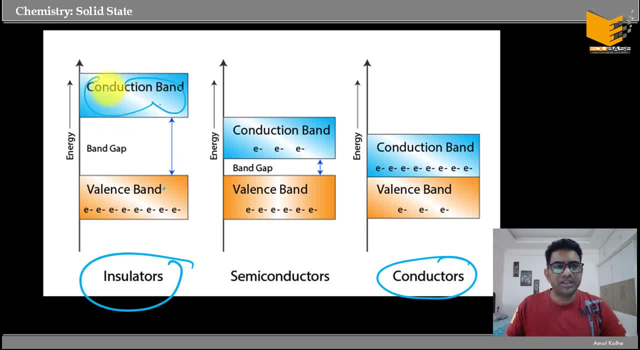 because at any given point electron can be in there. some electron can be there and you can have some conductivity, but that conductivity will be very less because there will be very less electrons. we will call it insulator, ok, so it is not equal to conductivity, so that 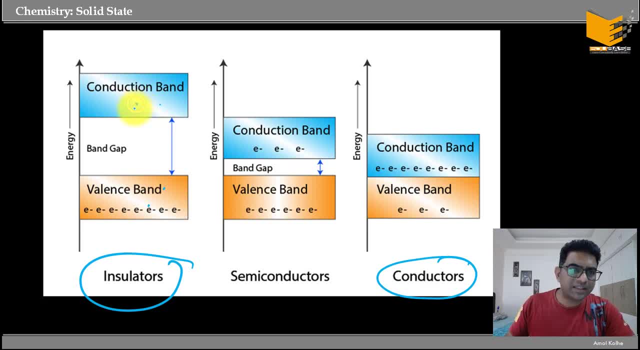 is called as insulator. so we can't go from valence band to electron conduction band. why? because the band gap, or forbidden gap, is there, so we can see it is very high. so here we will not get conductivity at all. now the third type is semiconductor. semiconductor will be in between of these two. ok, you can have a. 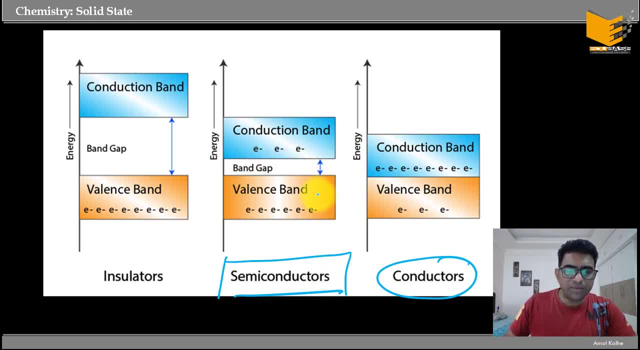 small gap and due to small gap, electrons can jump from valence band to conduction band. ok, and how much energy will it take will depend on the energy of this gap. how much is the energy of the gap? ok, how much the forbidden energy will depend on that, but the electrons 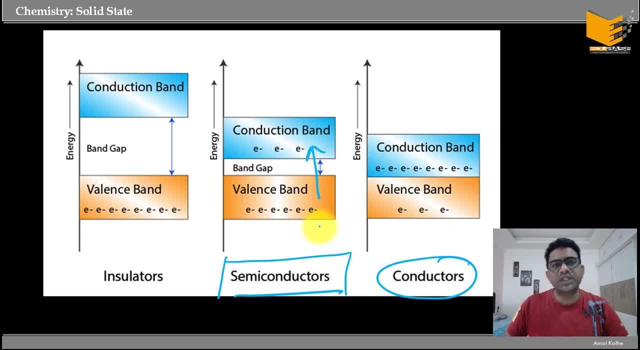 Electrons can go from valence band to conduction band and, due to the gap, there won't be many electrons here. There will be some electrons. that's why we will get some conductivity, and this is what we call semiconductor. In semiconductor the conductivity is less, but not negligible. 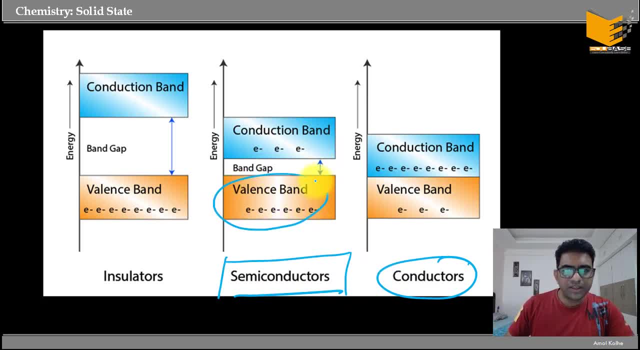 I hope that you have understood that electrons are going from valence band to conduction band, Jumping through this forbidden gap, and how much energy it will take will depend upon how big the gap is. It will depend on which material it is made of. 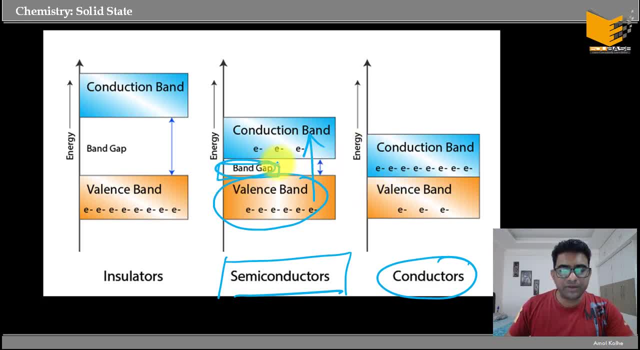 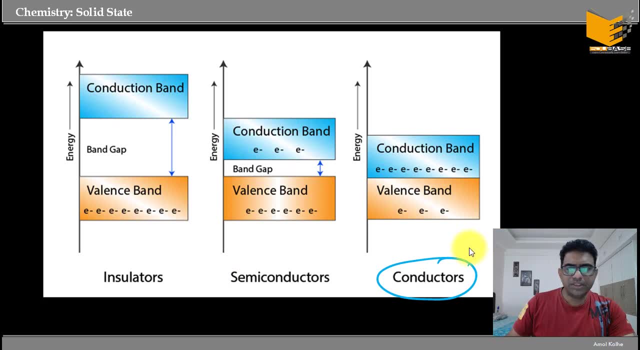 The band gap will be determined on the material type. The conductivity will be determined on the material type. I hope that this is clear. These are conductors, these are semiconductors and these are insulators. You will also get this in physics, so don't worry. 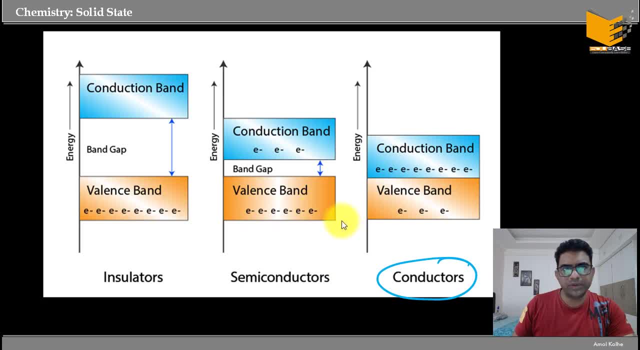 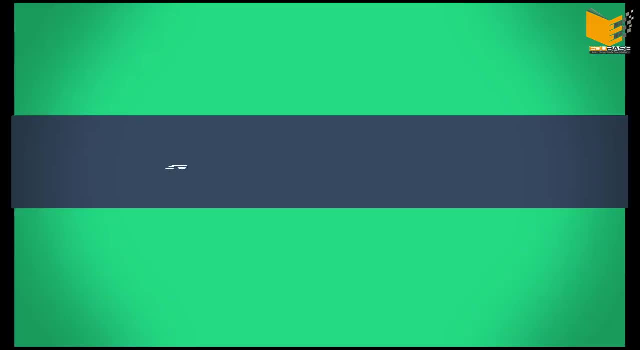 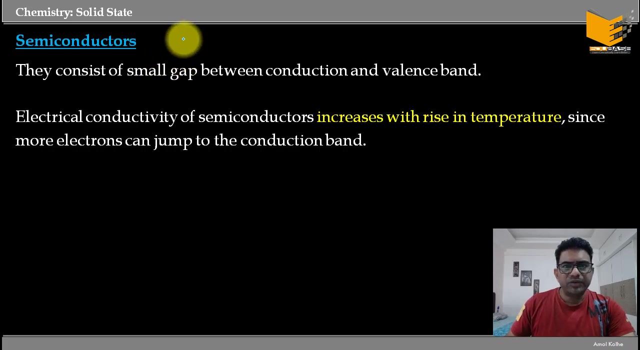 You will study this in more detail in physics. In chemistry, we study this from the perspective of molecule and orbital theory. We have done that. If you combine both in physics and chemistry, it becomes more sensible, Okay, Okay. so now let's look at semiconductors, because, remember we said, our focus point is semiconductors. 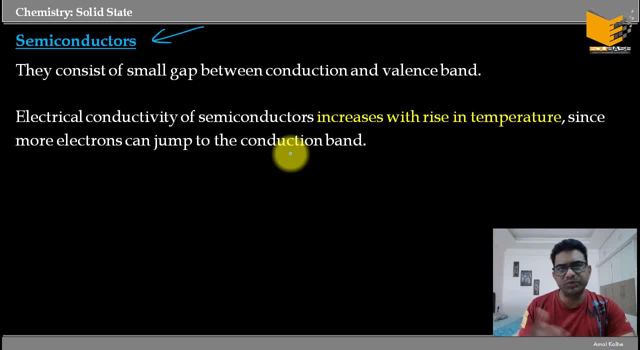 Conductors will come to you in physics. Insulators will also come to you in physics. Semiconductors come in both places. So semiconductors, they consist of a small gap between conduction and valence band. We just saw that. 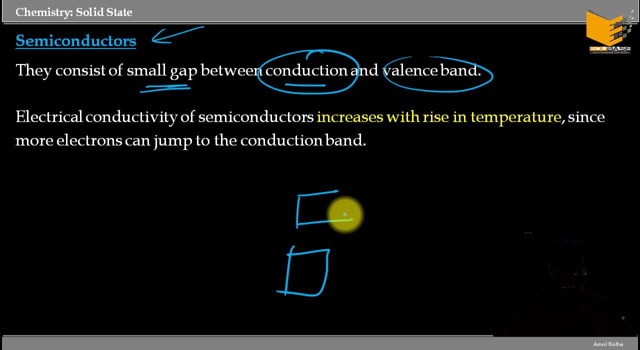 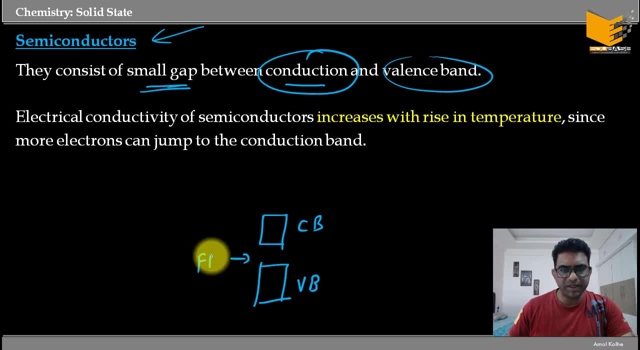 And the gap will depend upon that material. Okay, So this is valence band, This is conduction band And this is forbidden band. So electrons will be in valence band, Okay, And from here they will jump into conduction band. 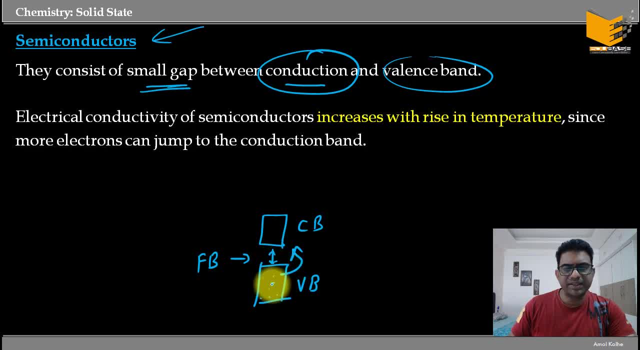 So how much energy will it take will depend upon this gap, And this gap will depend upon that element. Okay, So if I increase the temperature, then what will happen? Conductivity will increase. Okay, If I increase the temperature, then conductivity will increase. 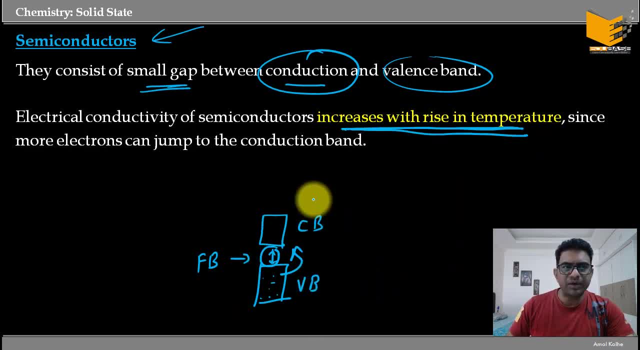 And that is with semiconductors. Okay, So electrical conductivity with semiconductors increases as we increase the temperature. Okay, Because here we are providing the energy required to jump. If we are providing energy in this case, then conductivity will increase. 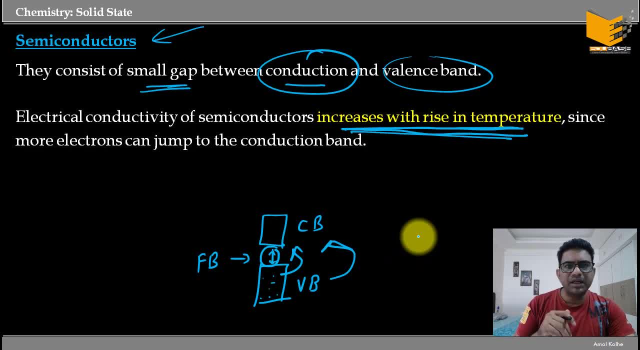 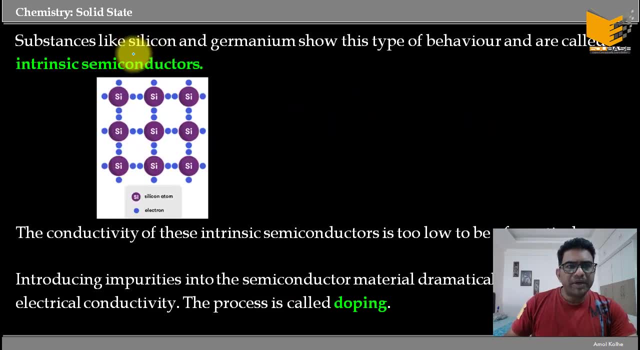 So keep in mind for semiconductors, when they provide energy, when they provide temperature, when they provide heat, then conductivity increases. So some compounds like silicon or germanium- You will remember that silicon and germanium are the heart of semiconductor technology. 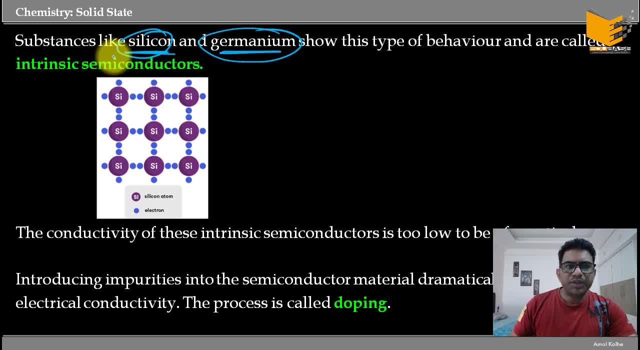 Basically, semiconductors are made from them. Okay, So these compounds, typically at natural state or normal state, they have some conductivity, So they are intrinsic semiconductors. Okay, Intrinsic semiconductor, There is some conductivity, Okay, 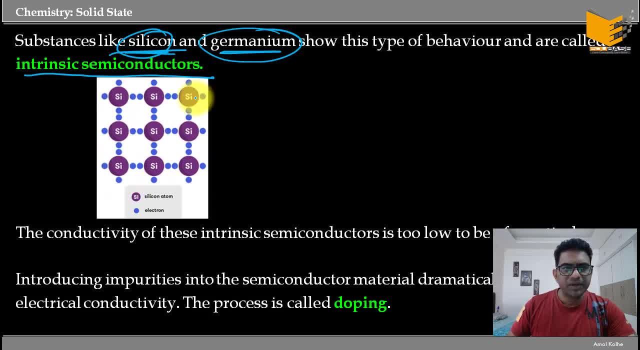 So here you can see the silicon network. Okay, Silicon network, And these are basically covalent bonds. You can see, silicon's valency is 4.. So you can see the network solid here. Okay, The blue dots, these are basically electrons. 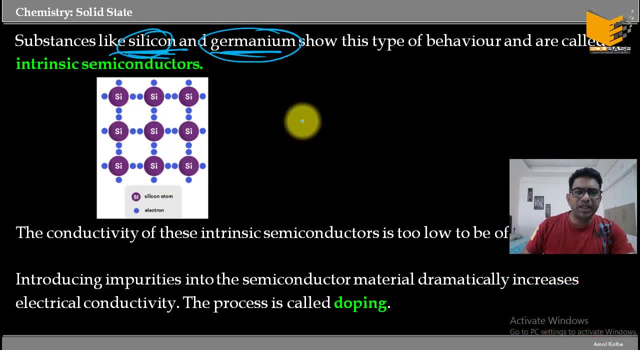 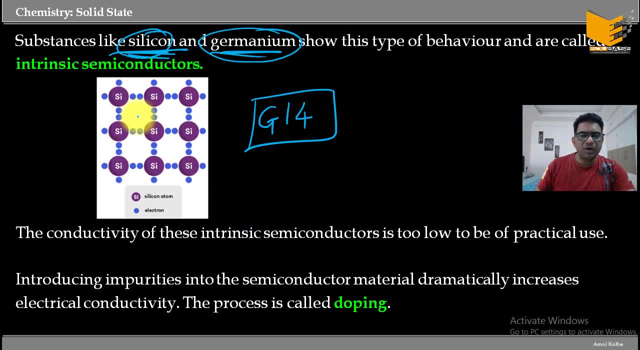 Alright. So silicon and germanium, They come in the same group, Both of them, They are in group 14. Their valency is 4. And both are intrinsic semiconductors. But this semi-conductivity of these, it is very less. 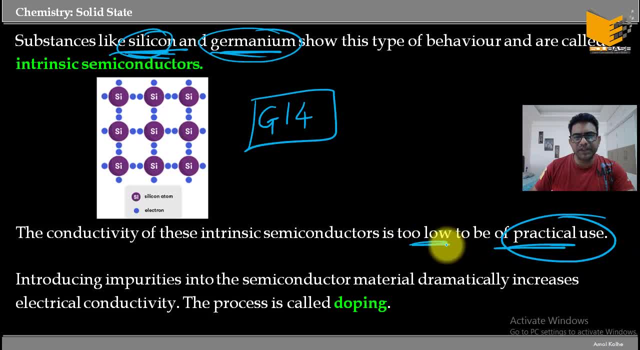 They cannot be brought into practical use. Okay, This is very low. Okay, Intrinsic semi-conductivity of these elements is very low, So we cannot practically use it. We will have to increase its conductivity, Isn't it? So how will we increase the semi-conductivity here? 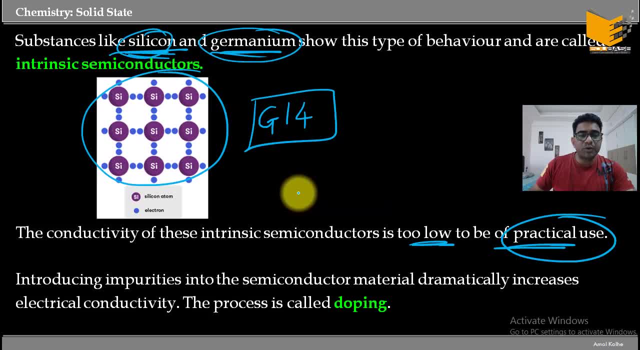 It is increased by a process called as doping. We increase it by doping- Okay, You must have heard this word more in sports. Okay, Doping is basically trying to increase the performance by taking some sort of enhancement inducing drug. Okay, Like steroids or any other drugs that sports people take to increase their conductivity. 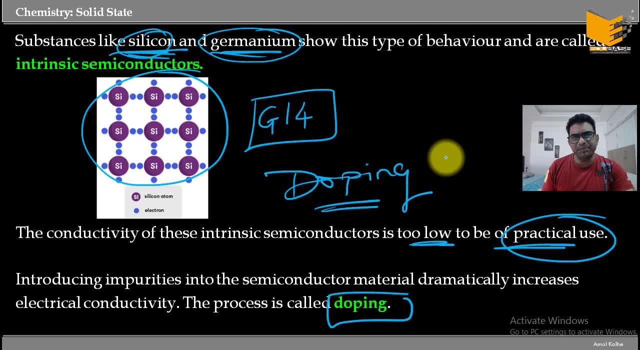 To increase their performance. That process is called as doping. Means we are adding some sort of impurity in our body, which is a drug, Isn't it? And because of taking this drug, our performance increases. So this is called doping. Similar process is used for these elements. 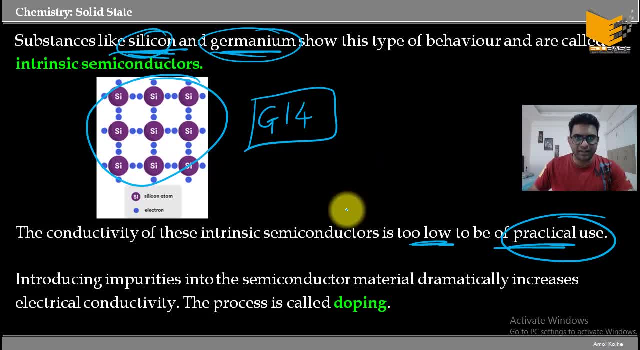 Okay, For semiconductors. So here we add impurities. Okay, This is a pure lattice structure of silicon, And if I add impurity in it, then its conductivity will increase. And what are we calling the process? Doping? 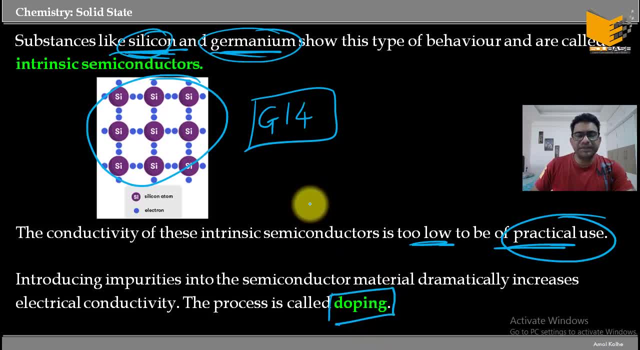 Okay, So what is happening with doping? Electrical conductivity is increasing Alright, And the more doping I do Means the more impurity I add in it, the more electrical conductivity it will increase, Isn't it? So we can increase the conductivity by adding some impurity. 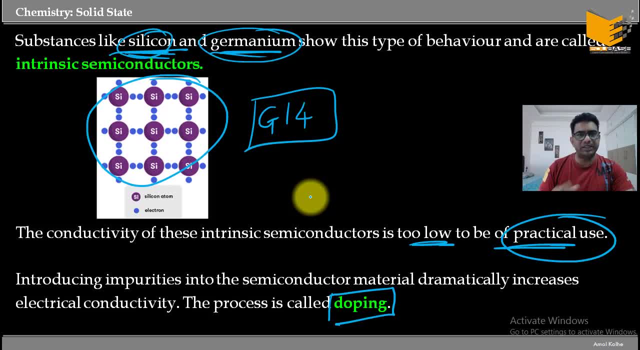 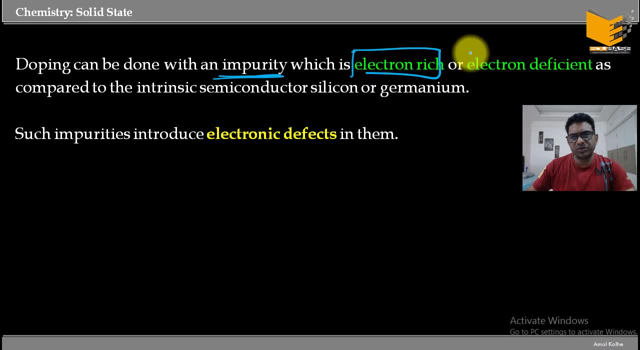 And if I I can control it, How much conductivity I need, I can increase its conductivity according to that. Okay, So I can control it. So we add two types of impurity: One is electron rich And the other is electron deficient impurities. 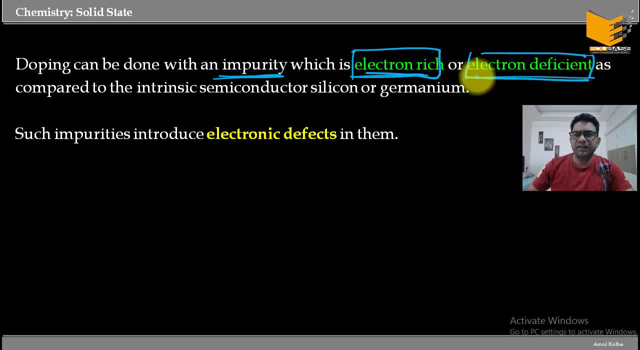 Okay, We add electron rich impurities Or we add electron deficient impurities in it. Silicon or germanium is our typical material in which we add impurities And due to these impurities, electronic defects will be created And due to electronic defects, conductivity will increase. 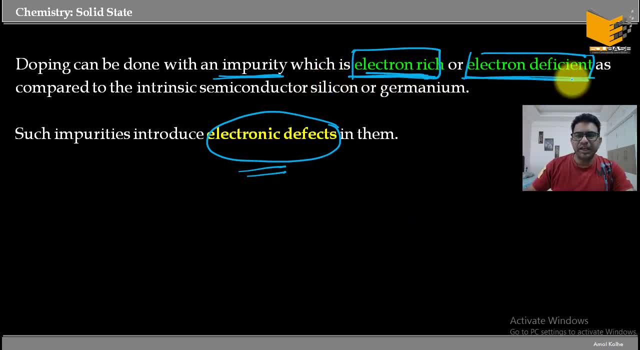 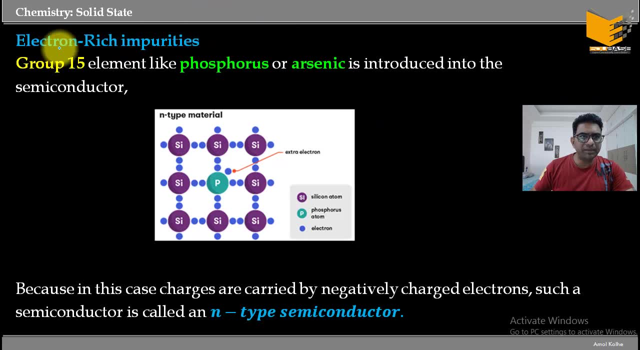 Okay, So we will see how conductivity increases. Now we will see what happens by adding these impurities. So first of all we are seeing electron rich impurity. Electron rich impurity means any element is adding impurity in it. of group 15 element. 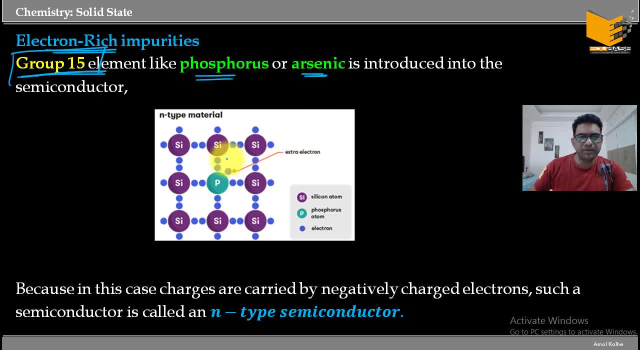 Okay, Like phosphorus or arsenic. See, I have silicon network And in that I have added phosphorus impurity or arsenic impurity. Okay, So now what will happen? See phosphorus or arsenic. This is element of group 15.. 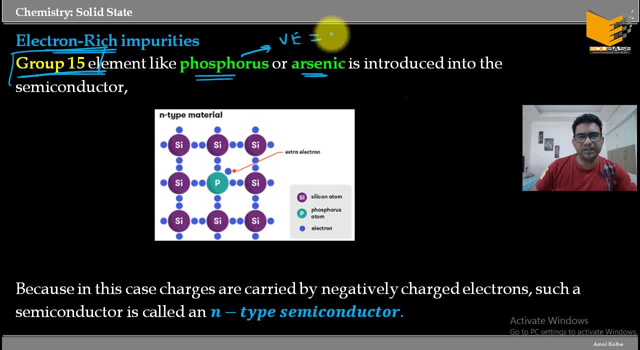 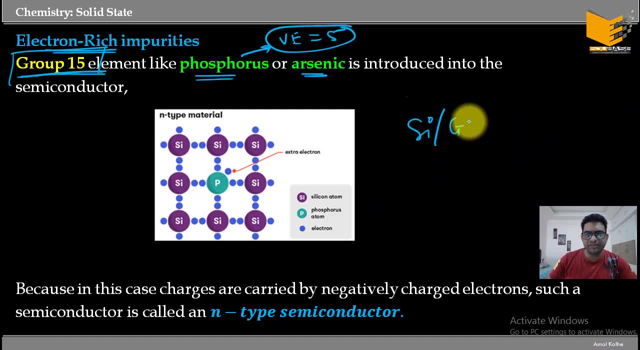 So in these valence electrons is equal to 5. 5 valence electrons. Okay, And silicon, or silicon, or germanium, Germanium, This is element of group 14. And in these valence electrons is equal to 4 valence electrons. 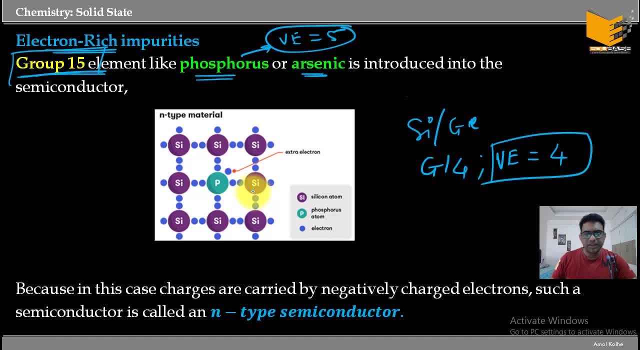 Okay. So these 4 electrons are using silicon, But when we add phosphorus, impurity or arsenic impurity. So because they have 5 electrons, 4 electrons will be used in bonding, Okay, And 1 electron will be left. 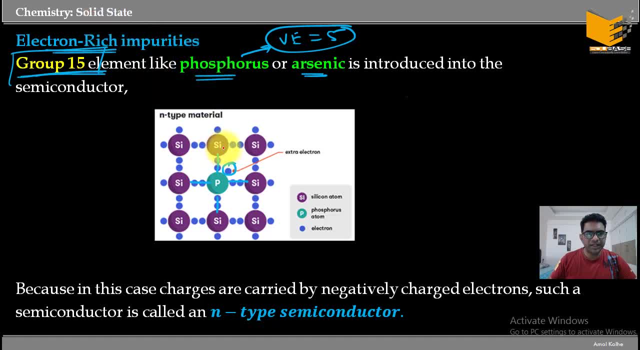 And that is going to have a negative charge. Okay, So this electron is an excess electron. Many impurities will be present like this: Okay, As compared to the entire network, we are adding very less impurity, But obviously there are going to be few thousand of these impurities. 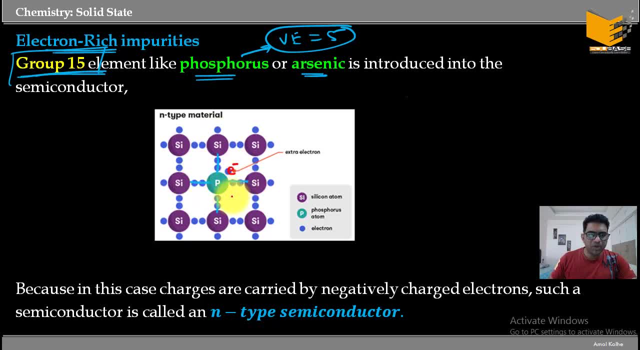 So now what will happen? Here we are showing only one. Keep in mind Now what will happen, Like if I have joined it to the circuit. Okay, So in this case, this electron will move Because this is a free electron. Okay, 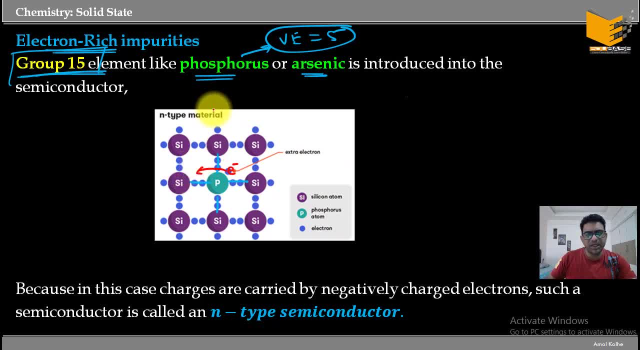 So electron will move And current, we say exactly, flows in the opposite direction. Okay, If the direction of electron is this, If electron is moving in this direction, Then current- we say by convention, is moving in the opposite direction. Okay, So here we are getting conductivity because of that free electron. 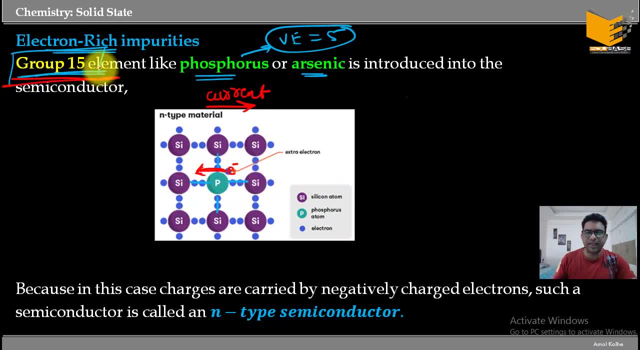 When we add impurity of this group 15. So we are adding excess electrons in it. Okay, And these electrons move to give us conductivity. Now, here on the electron, there is negative charge And because of negative charge we call these semiconductors as n-type semiconductor. 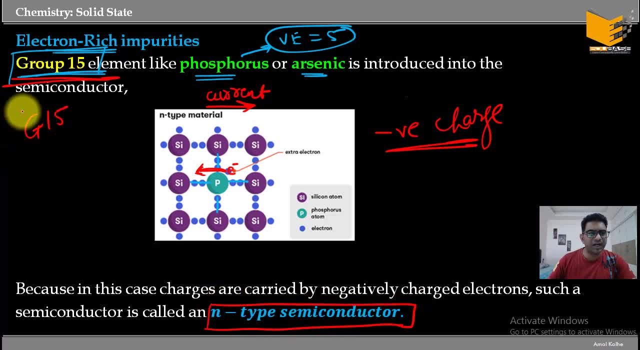 So what we have to keep in mind, If I add impurity of group 15.. Okay, Then we are getting n-type semiconductor. Okay, In the same way, we can add electron deficient impurities In this. we have to add elements of group 13.. 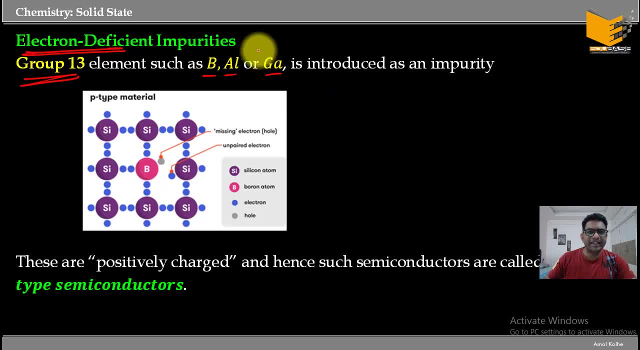 Like boron, aluminium Gallium, Here there are three valence electrons, So there are only three valence electrons, Means one electron is less as compared to silicon, Isn't it? So what will happen here? Like I have added boron here, 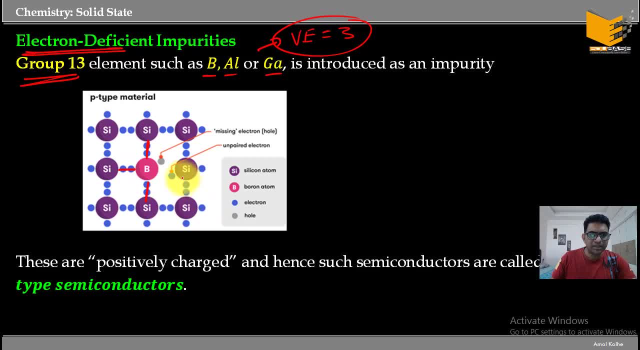 So it will make three bonds, But it cannot make one bond, So this electron will remain free Of silicon At the same time. There will be a gap here. That is a missing electron. We are calling it as hole, Okay. 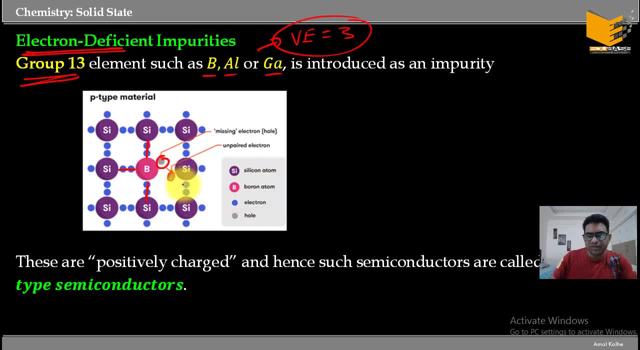 The electron is actually missing From that position, So that's why there cannot be a bond here. This unpaired electron will remain with silicon. Now what will happen When I will put it in the circuit? So the electrons will jump here. 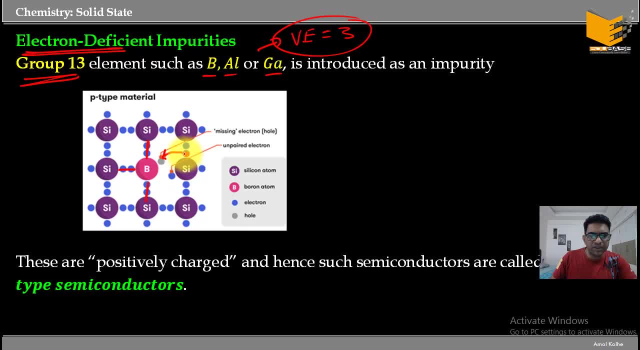 If it is jumping here, Then a hole will be created here. Okay, Then the next electron will jump here. Okay, So a hole will be created here. So see, electrons are going in this direction. Okay, The movement of electrons is in this direction. 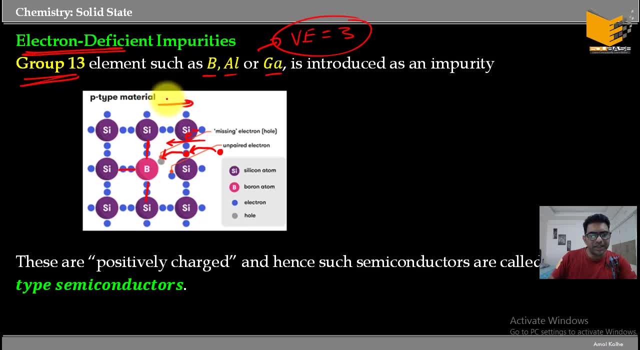 Means the flow of current will be seen in this direction. So this will be the flow of current And if you see in this direction, Then the hole is moving. Okay, The hole is moving in that direction. What is happening in this case? 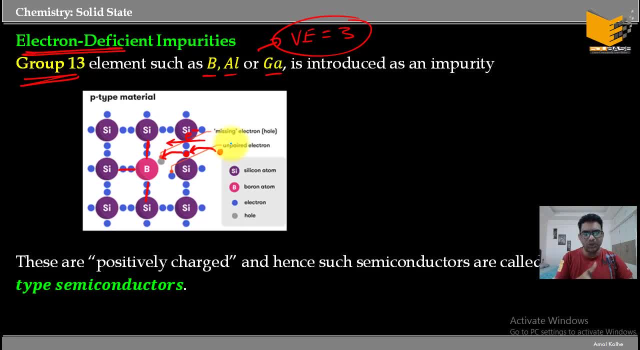 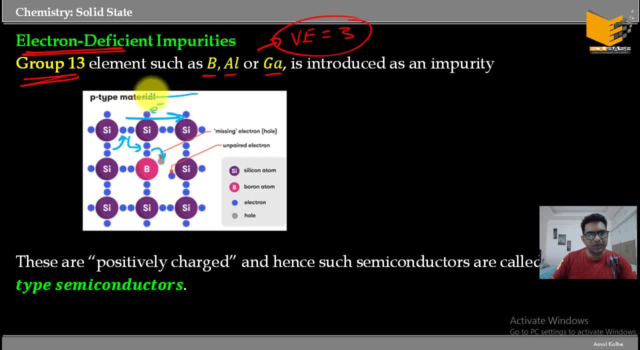 So in this case The electrons are moving in that direction, So current will be in that direction And hole is moving. Because if we keep holes, If the electron is here, Here hole is creating, Then hole is creating here, Then here hole is going in this direction. 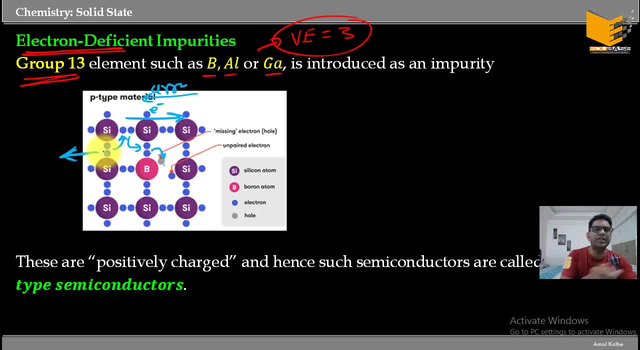 So hole is? It seems like the hole is moving in In the same direction as that of current. Okay, Hole is not actually moving The electrons. that is jumping into the hole. that is jumping into the hole, but if we see it will feel like the hole is moving. so here. 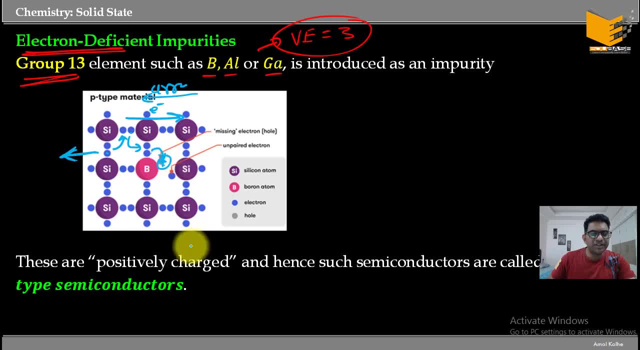 basically, it seems like due to electron deficiency, there is going to be a positive charge, alright, and due to positive charge or due to assigning, it is going to be a p type semiconductor. so keep in mind that if we use elements of group 13 as a doping agent, then we will get p type. 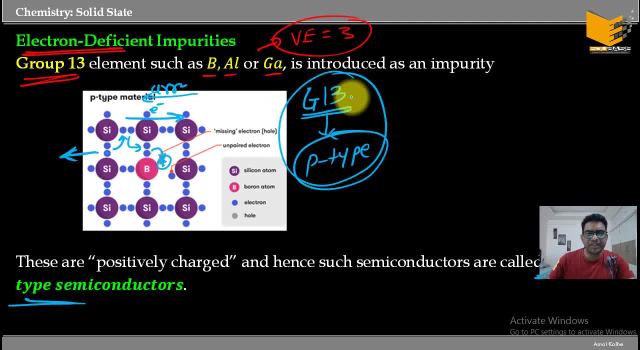 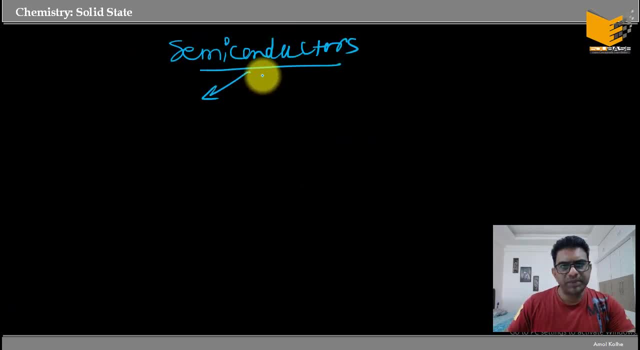 semiconductor got it. so p type semiconductor is available by group 13 elements. so summarize this: we have semiconductors, we get p type and n type. ok, p type semiconductor can be found when doping주 Só group 13 and n type when dopingungás with group 15 элемент. 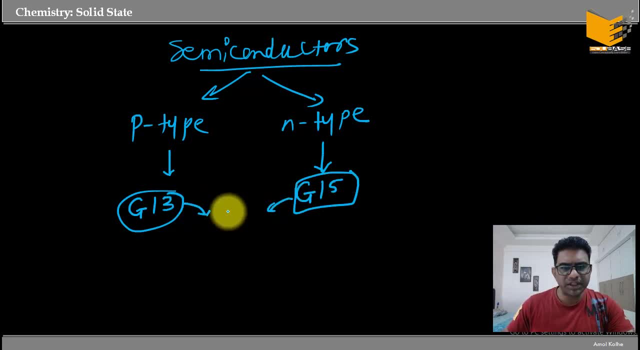 ok, and we are doping group 14 elements. so in group 14 we use silicon and germanium. so often question is asked in exam that if I add arsenic then which type of semiconductor will I get? so which group element is arsenic? 15? 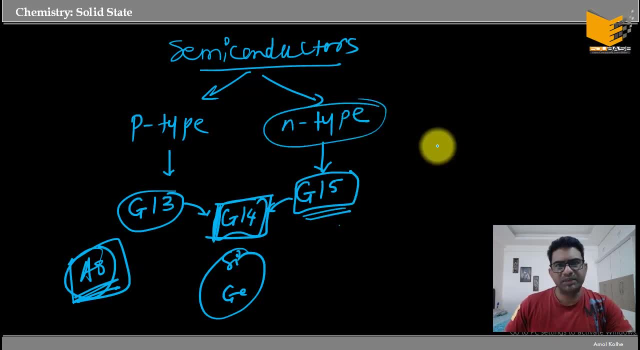 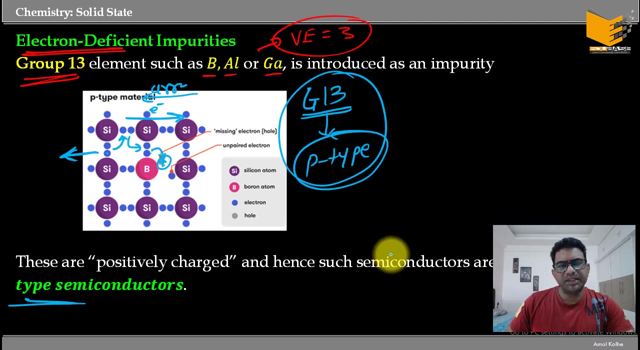 if I am adding 15 element, then which type will I get? n type. if I add aluminium, then I will get p type semiconductor, because aluminium is group 13 element. so you should know all these things understood. so this was about semiconductor. now we will see magnetic properties. 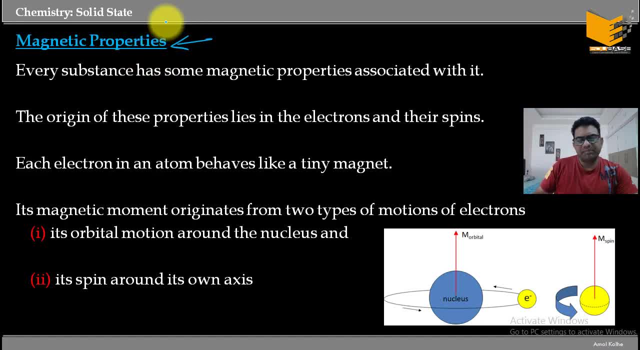 ok, let's talk about magnetic properties of solids. this is a simple concept. again, this is going to be in physics also nothing to worry about, but if you do it properly here, you will understand it better. ok, be careful. every substance has magnetic properties associated with it. this magnetic property is measurable or not measurable. 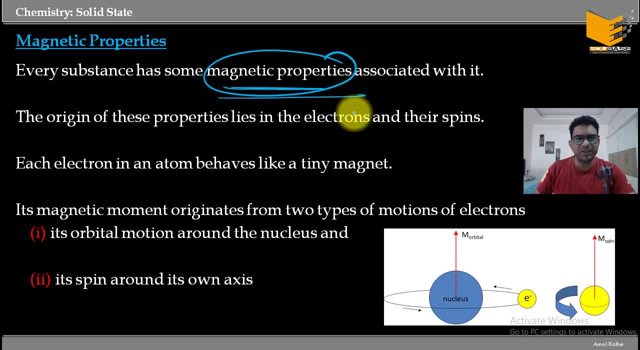 that is something that is a different issue. ok, but magnetic properties are associated with it. ok, and where do magnetic properties come from? where do they originate? because of the electrons. electrons, because there are spins of electrons from these spins. sorry, magnetic properties result from these spins. 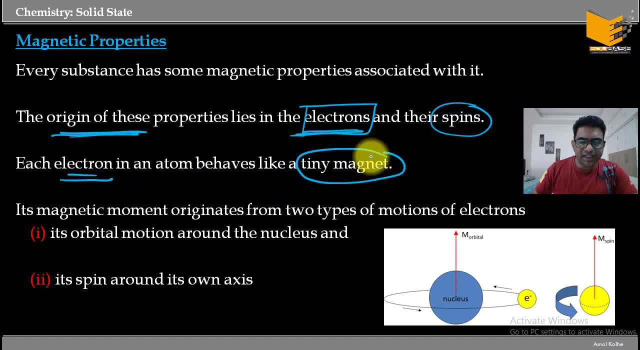 ok, each electron behaves like a tiny magnet. ok, whatever electrons are there, those electrons, basically they are a tiny magnet and that's what creates the magnetic field. ok, now see, electrons show two types of motions. one is orbital motion and the other is spin. in orbital motion, there is a nucleus and electron is revolving around it. 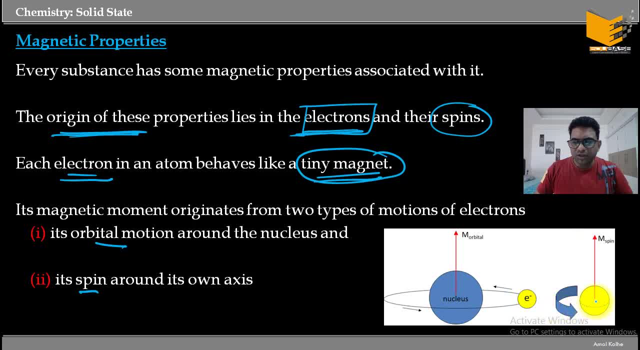 so this is called orbital motion. second is spin. electrons are rotating in their surroundings, only this is basically like earth: earth is revolving around the sun and earth is rotating around its axis. so here, electron is rotating around its axis. ok, so this is orbital motion, this is a spin motion. 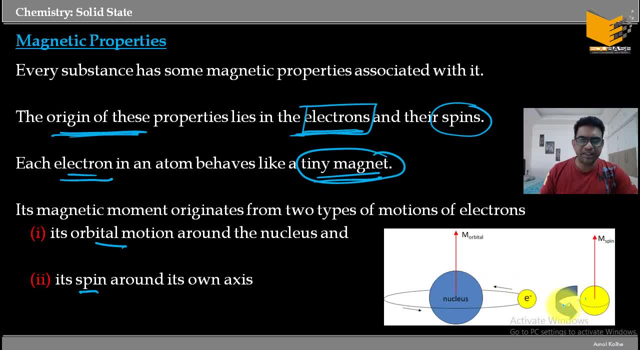 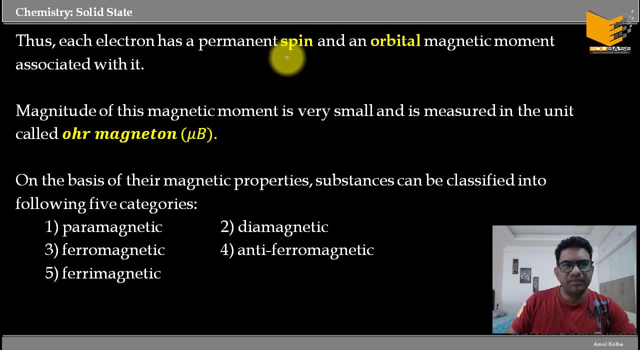 so because of both of these, magnetic moment is generated. ok, so magnetic moment is generated because of the orbital motion around the nucleus and spin around the axis. so because of these two motions, magnetic moment is created. so these motions we we call magnetic moments: spin magnetic moment and orbital magnetic moment. 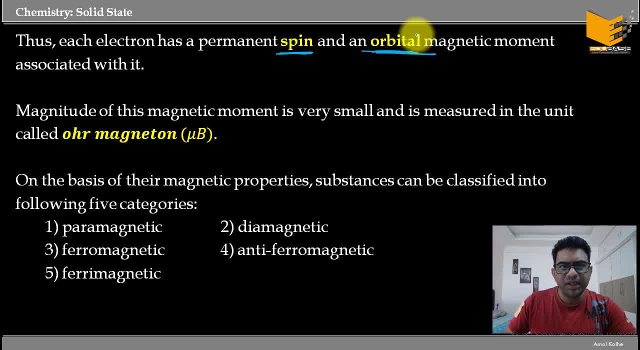 ok, so we have spin magnetic moment and orbital magnetic moment. generally, the orbital magnetic moment is negligible. we don't count it, ok, the measurable one is usually spin magnetic moment. ok, so we will talk about this. but even in that case the magnetic moment is very small because- remember- 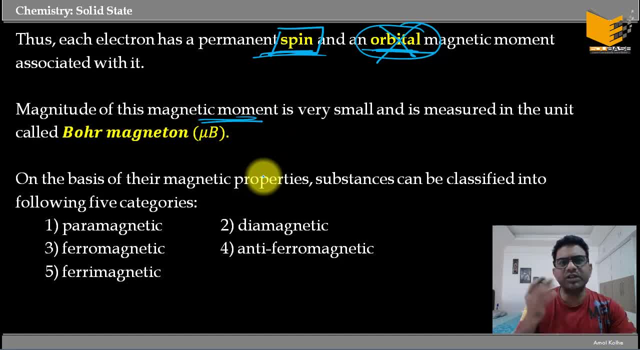 the magnetic moment of one of the tiniest particles right, the magnetic moment of electron. so the magnetic moment of individual electron is very less. we measure this in Bohr magneton. its unit is nu b. ok, we measure in Bohr magneton, we don't actually do any calculations with it. 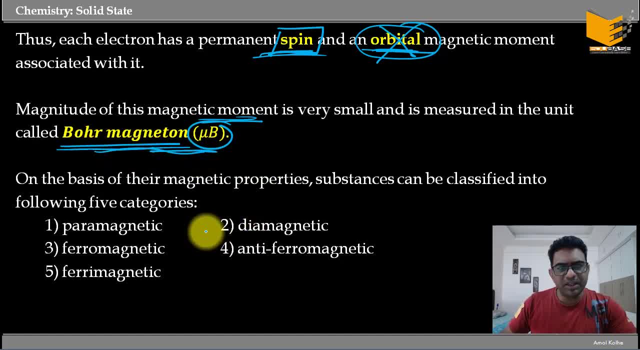 there are calculations in physics, but not in chemistry. ok, at least not at this point. when we see d block or coordination chemistry, there is some calculation, but the magnetic moment that is coming, that is because of the spin of the electron, ok, because of orbital. the result is: 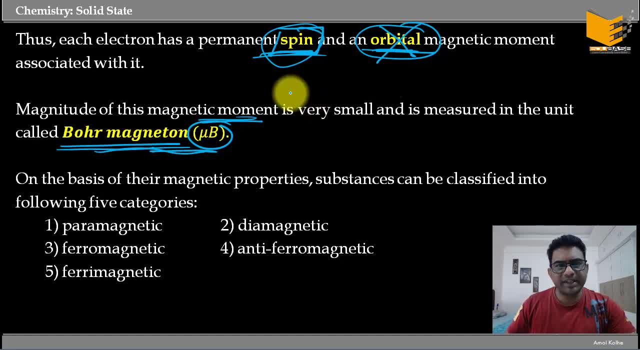 orbital magnetic moment: that is very small, negligible, so we are neglecting it. spin magnetic moment: that is measurable for us and we measure it using Bohr magneton. ok, so the magnetic property. we can classify it in five ways. one is paramagnetic, diamagnetic, ferromagnetic. 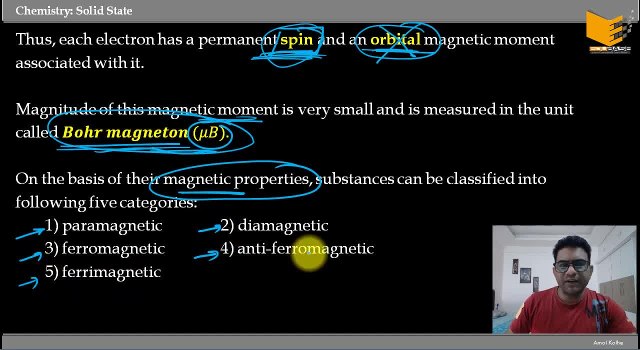 antiferromagnetic and ferrimagnetic. these are five types of magnetic compounds. ok, so we will discuss these five alright. paramagnetic- you might have known it till now. paramagnetic and diamagnetic: we have talked about it many times, so I am sure you know what. 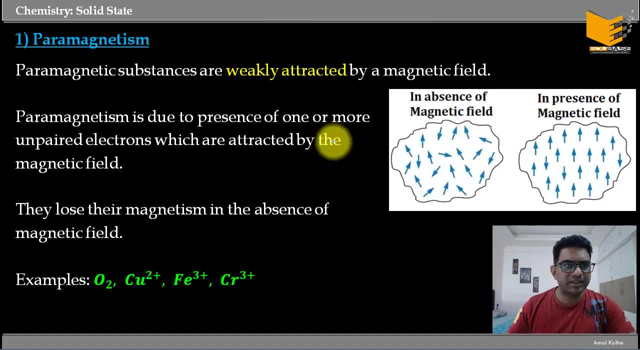 paramagnetic and diamagnetic is ok. still, we will discuss it once. paramagnetic substances: these are weakly attracted by the magnetic field. keep in mind, they are weakly attracted. they are not strong enough, they are not strongly attracted, they are weakly attracted. so here see these electrons. 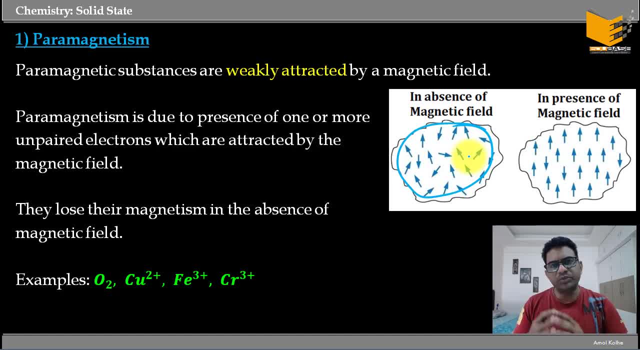 ok, these electrons, whatever element you are taking, whatever compound you are taking, there are electrons, isn't it? and these electrons, if there are unpaired electrons, so these are not going to be forming bonds. ok, these are unpaired electrons, they are basically not connected to anything. so the spin of these? 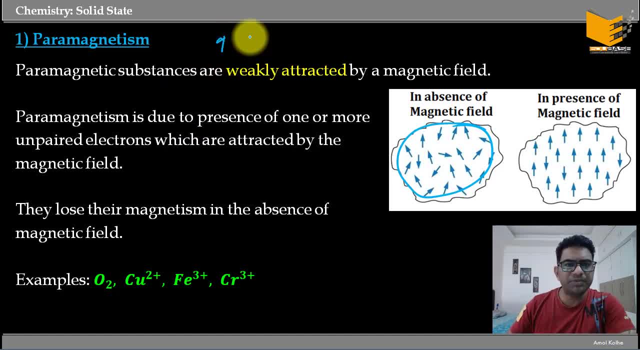 ok, there are two spins, if you remember: up spin and down spin, isn't it? so the spin of these, that is randomly oriented. ok, in absence of, in absence of any magnetic field, so in absence of any magnetic field, the spins of these, these are going to be randomly oriented. 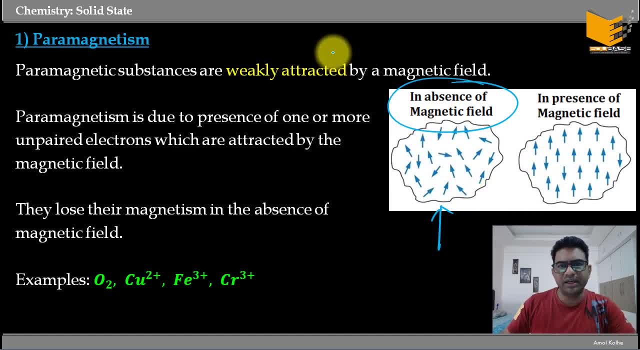 and because of this, the net magnetic moment that we will get, that is going to be zero in this case. but if I bring a magnet near this compound, so these, the spins of these electrons, they will be oriented either in the same direction or in the opposite direction. 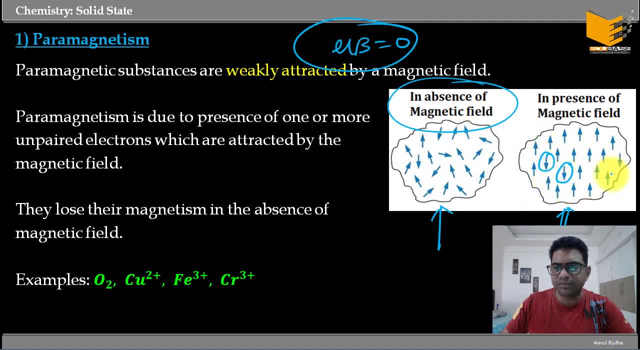 ok, see here some compounds, some spins. they are in the opposite direction. alright, so most of the spins are in the same direction. there are few spins that are in the opposite direction, so it is possible that all of them spin in the same direction, or some at the direction of the magnetic moment. 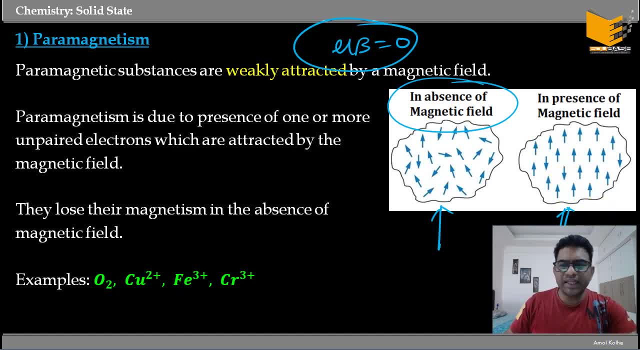 and some are opposite to it. but, in any case, here we can see the order, isn't it? and because of that, the magnetic moment that we will get here, that is going to be not equal to zero. ok, so this magnetic moment that is going to be not equal. 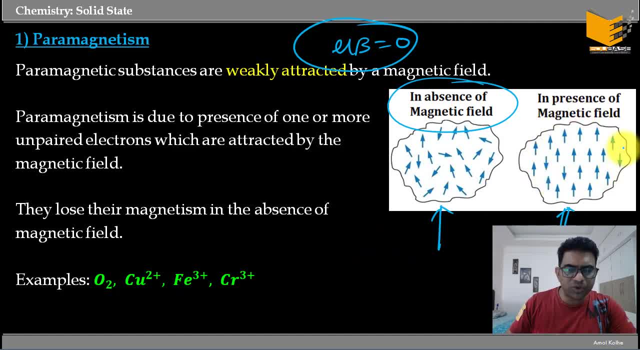 here we will get some magnetic moment, but as soon as I remove this external magnetic field it will revert back to its disordered condition. ok, so essentially what is happening, that disordered condition- is that, in absence of external magnetic field, no magnetic moment as soon as I bring. 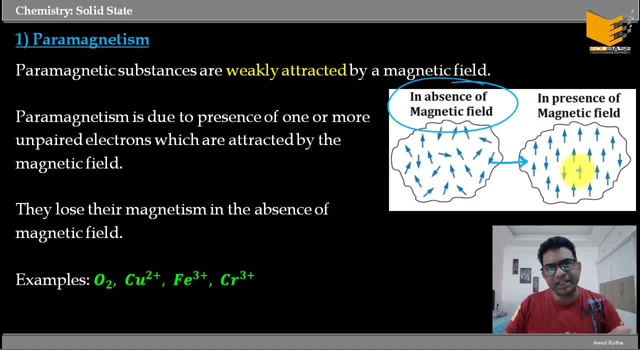 the magnet. it is going to get oriented and you get some magnetic moment. magnet is removed, it will revert back to its original condition, so we can call this temporary magnetism. it is not a permanent magnetism, it is a temporary magnetism and it is very weak. 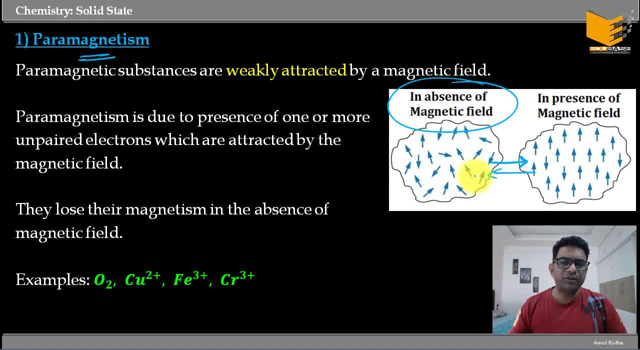 ok, so as soon as you remove the external magnetic field, they will lose their magnetic property. ok, so that's what we are seeing in the video, so we can see that. we can see that there is some magnetic element around this side. that is the surface of the. 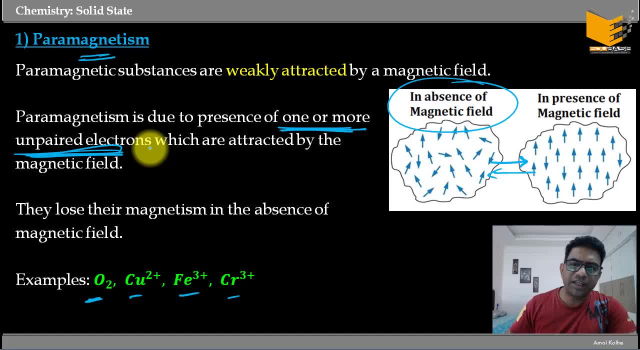 magnet. now we will see that if the magnet keeps and we will not get any net magnetic moment understood. so what happens is that if there is a paired electron, then their spins are paired, so the spin of this will be canceling this and canceling this. but if there is an unpaired electron, 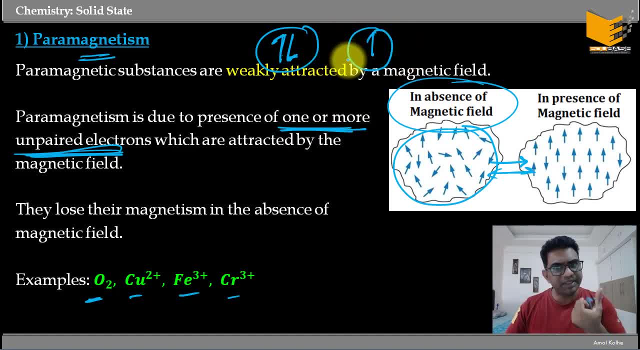 then this is not getting cancelled. it will have an inherent spin. but because all these electrons are randomly oriented, the net effect is that we don't get any spin. so in absence of magnetic field, there is no magnetic moment. but as soon as we get the magnet, they will be aligned and show us the magnetic property. 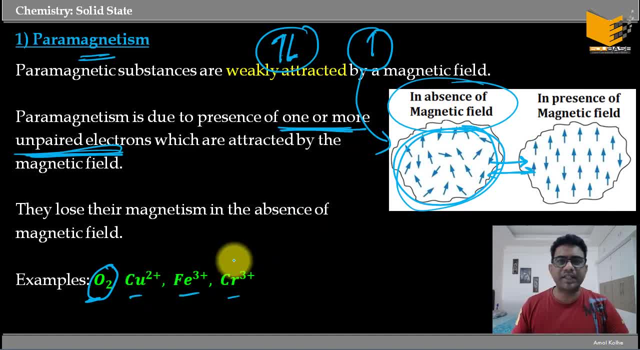 we saw that in oxygen there are two unpaired electrons. we had drawn a molecular orbital diagram of this. similarly, you can draw electronic configurations of these elements and you will see they will have at least one unpaired electron and that's why they are paramagnetic clear. 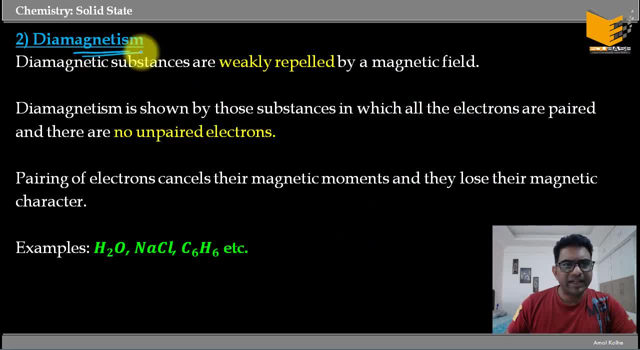 the next thing we are seeing is Dimagnetism. we will call the compounds that we will show Dimagnetic compounds. these are called. these are actually weakly repelled by the magnetic field. paramagnetic compounds were weakly attracted and dimagnetic compounds are weakly repelled by the magnetic field. 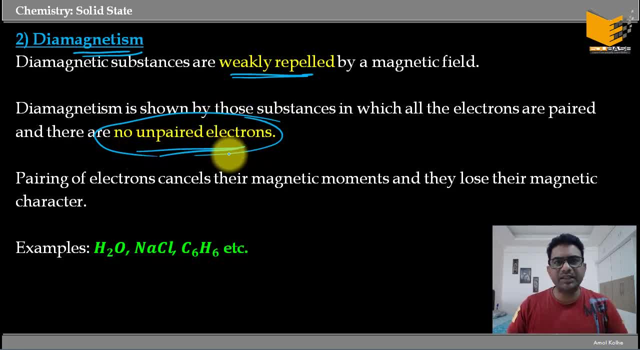 they don't have any unpaired electron. all the electrons here are paired. because of being paired they don't actually have any inherent magnetic field. so because of this they are called as dimagnetic and if I take a magnet near it then these compounds will be repelled. 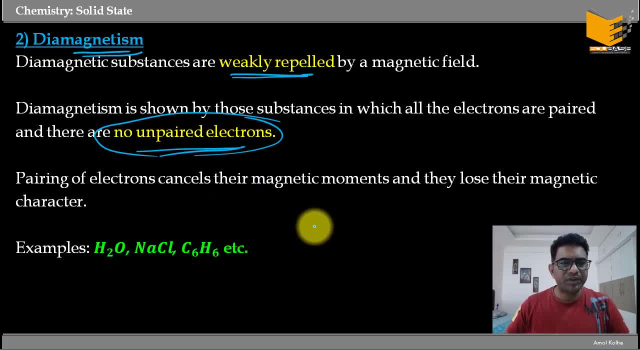 by the external magnetic field. ok, so because of being paired, the magnetic moment of all the electrons gets cancelled. I told you this earlier and that's why you don't get any magnetic field. examples: water, NaCl, benzene, basically any covalent compound in which covalent or ionic compound 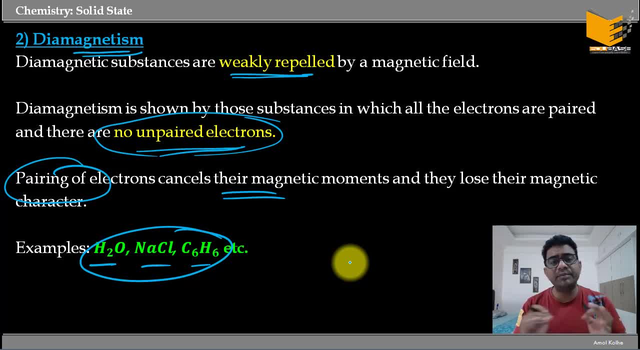 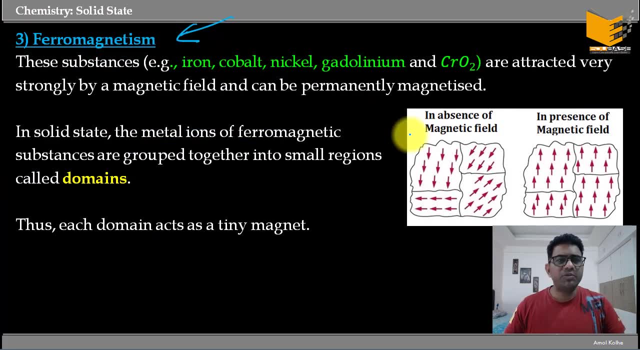 in which all the electrons are paired and there is not even one unpaired electron. such a compound will be dimagnetic. is it clear? third is ferromagnetism. ok, ferromagnetic compounds. these are called permanent magnet. these compounds show permanent magnetism, for example, iron, cobalt, nickel, gadolinium, chromium oxide. 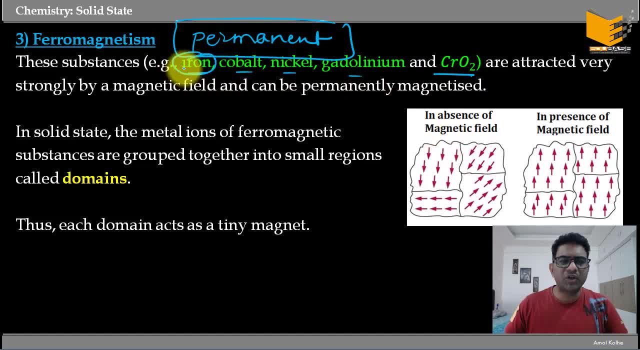 so how are all these compounds? ferromagnetic iron is the most common example of this. ok, we also use cobalt. this also shows permanent magnetism. alright, in this there are domains, means all the electrons, group of electrons. they act as a domain, so these are the domains. 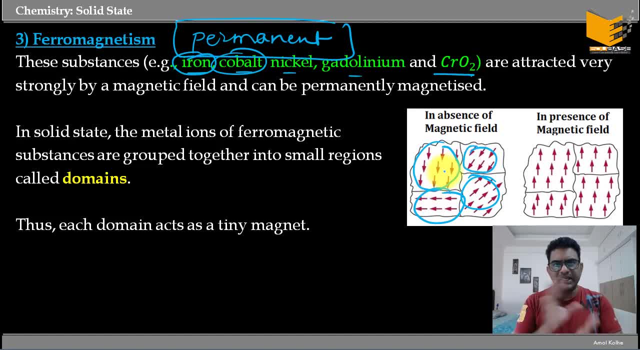 so what is happening in this? the ions of metal, they form a kind of domain. so the unpaired electrons will form a domain of them and these are organized in domains in absence of magnetic field. ok, so see, this domain's magnetic field is here, this domain's is here. 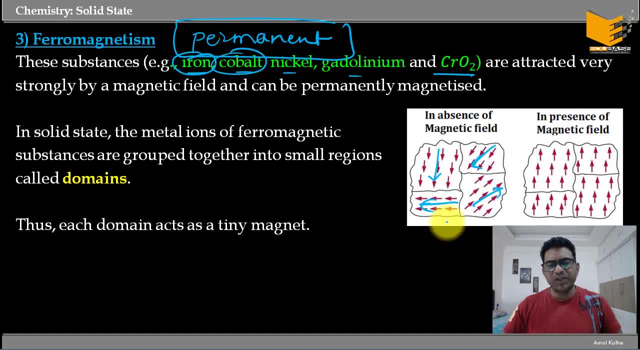 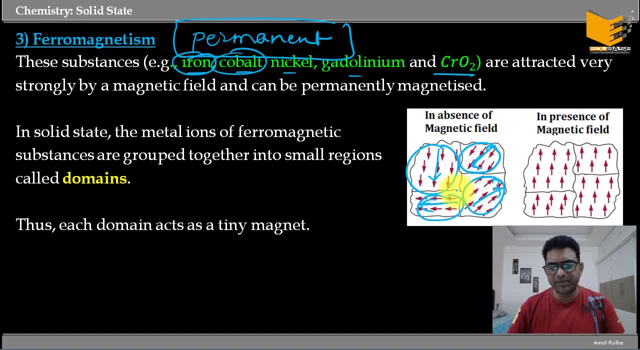 of electrons. they have a group, they have a group and they have a group. now, how does this happen? no one knows. basically, because you know that is their inherent property. ok, this is their inherent property and this is how they behave. ok, there is no plausible explanation for that. 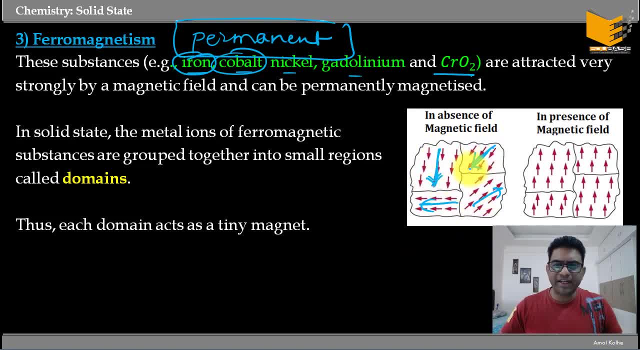 so these domains, their net magnetic field, we will see that. so they are again randomly oriented. so the magnetic moment of this that is going to be zero. ok, but if I bring an external magnet to this, so all these domains will align with that magnetic field and in this, 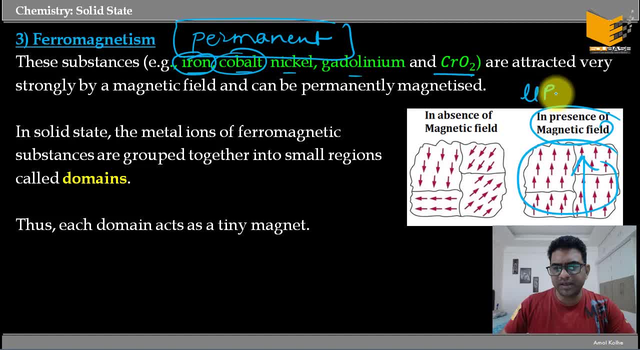 magnetic moment will come, ok. so in this case bohr magneton is not equal to zero, ok, but even if I remove the magnet, so it will not go in the reverse condition, it will be permanent. their domains will be aligned, ok. so this is what we call. 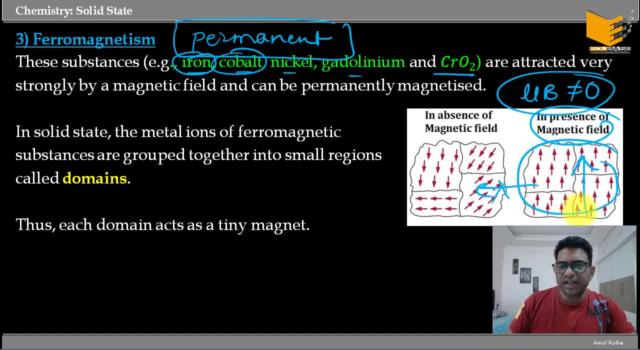 magnetism cause, isn't it in iron? in the same way we put a magnet, if you put a magnet in an iron plate, if you put a magnet in an iron plate, then in that plate also magnetism comes, ok, isn't it? and that is what we call as. 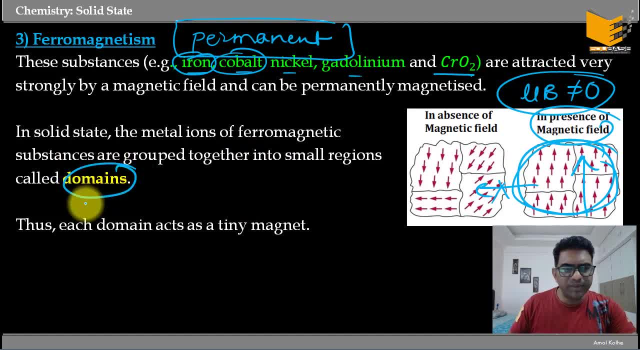 you know, creating magnets. keep in mind: in this, domains are behaving which is very similar to paramagnetism. there electrons are behaving independently. here electrons are behaving in groups. that's all ok. so each domain is basically like a tiny magnet, and in external magnetic field they get. 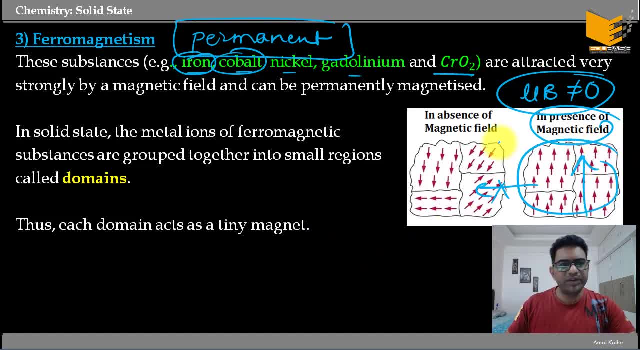 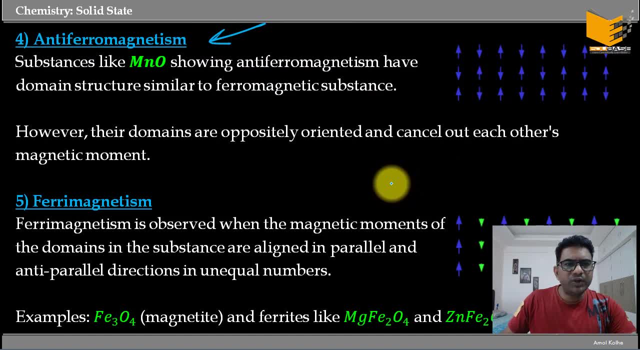 aligned with the external magnet. ok, and you get ferromagnetism examples. keep in mind: this one is anti ferromagnetism- ok, anti ferromagnetism. its example is manganese oxide- ok, this is also like ferromagnet, very similar to ferromagnet- ok. 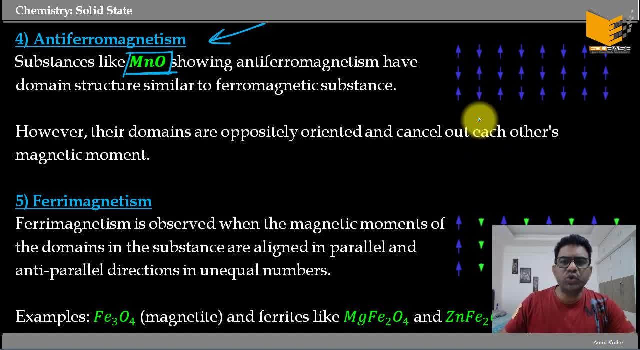 but in this, domains, domains are coming. in this, too, domains are coming, but domains will be exactly opposite. ok, so here the domains, their magnetic moment. that is equal and opposite. so, because of being equal and opposite, the net magnetic moment that you will get, that is going to be. 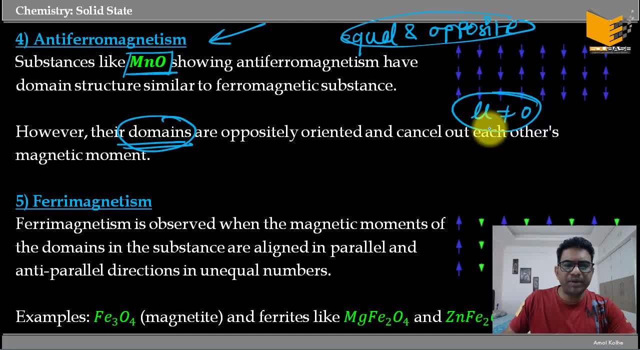 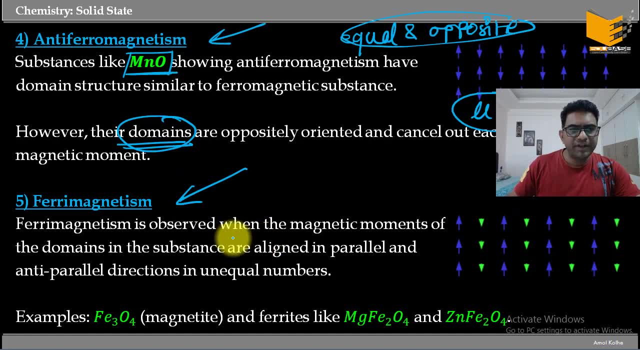 zero. ok, so here the net magnetic moment is zero, and the last one we have is ferrimagnetism. ferrimagnetism examples: see some oxides: iron oxides- these are ferrites. ok. mgfe2, o4- whatever its chemical name is ok. magnesium ferrite. 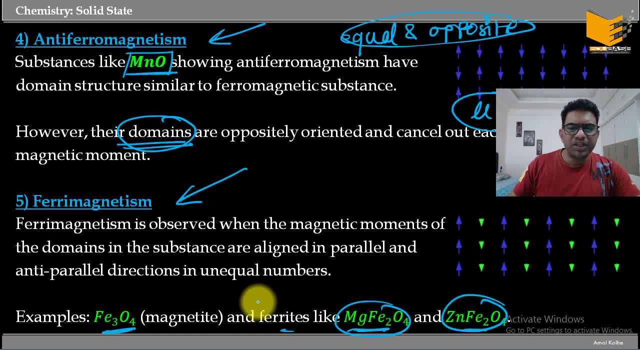 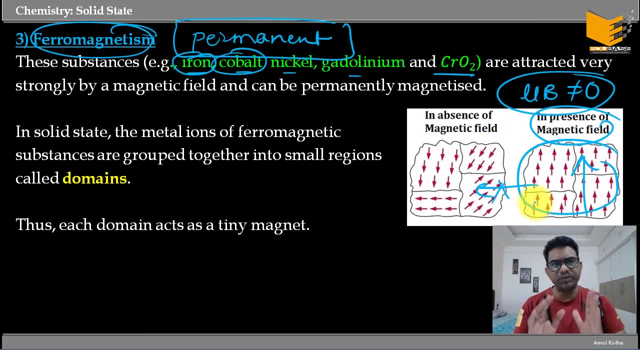 or zinc ferrite, so these are ferrites. ok, so these compounds, these show ferrimagnetism. ferrimagnetism is similar to antiferromagnetism. ok, see, in ferromagnetism all the domains, ok, in this one, all the domains align in one direction. 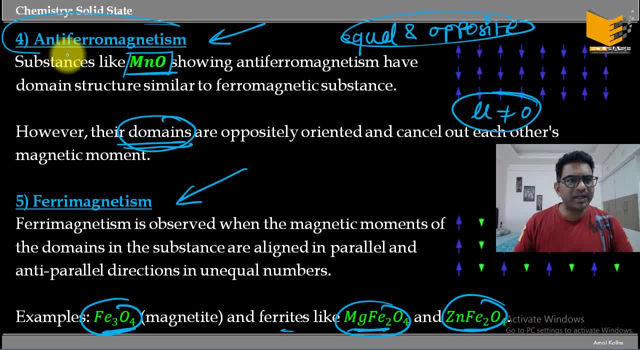 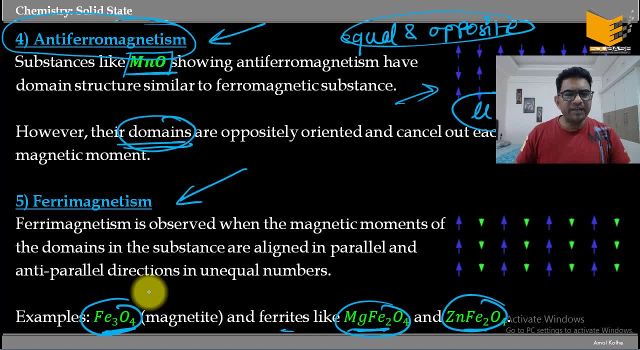 in external magnetic field. in antiferromagnetism they are equal and opposite. that is why the magnetic moment is zero. in ferrimagnetism they are opposite, but not equal, unequal and opposite. so because of this we will get some magnetic property ok in ferrimagnetism. 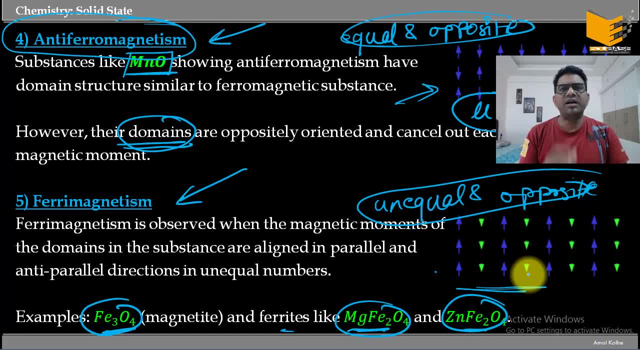 we will get some magnetic property in antiferromagnetism. we will not get, even though there are unpaired electrons, even though there is a property that could result into magnetism, but because of being equal and opposite, we don't get any magnetic property. ferromagnetism: